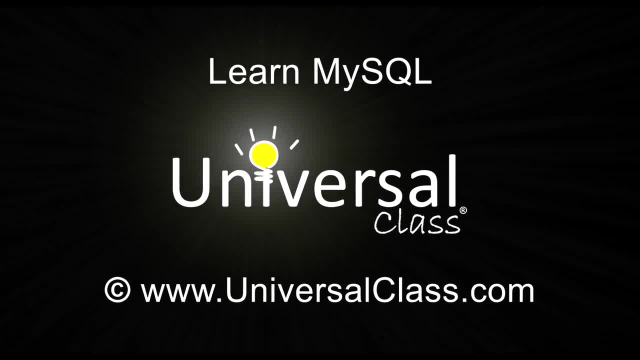 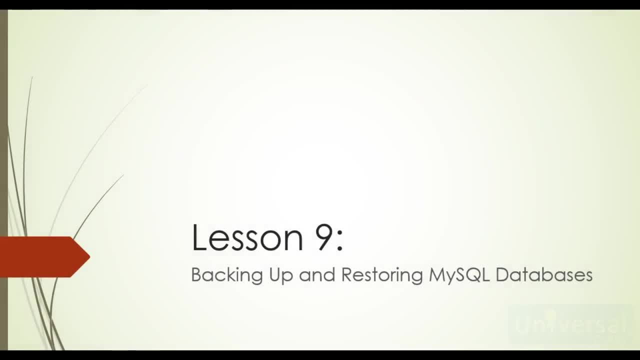 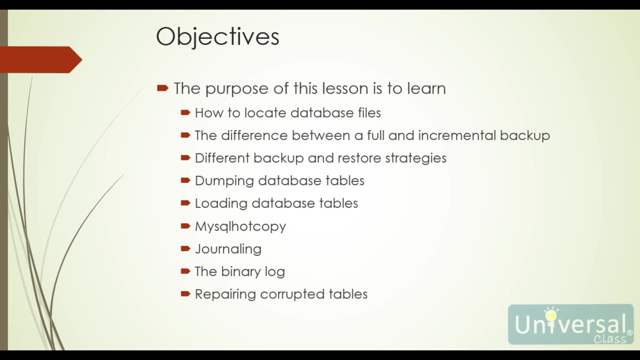 The purpose of this lesson is to learn how to locate database files, the difference between a full and incremental backup, different backup and restore strategies, how to dump database tables, how to load database tables, how to use MySQL, Hot Copy, journaling, the binary. 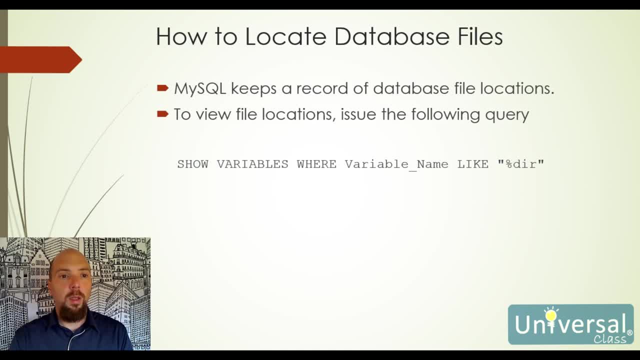 log and how to repair corrupted tables. The first part to being able to do backups is to know where your files are located. So to find the files, you can simply issue a command, And what happens is when you first launch MySQL, it reads in the contents of a configuration file and that configuration 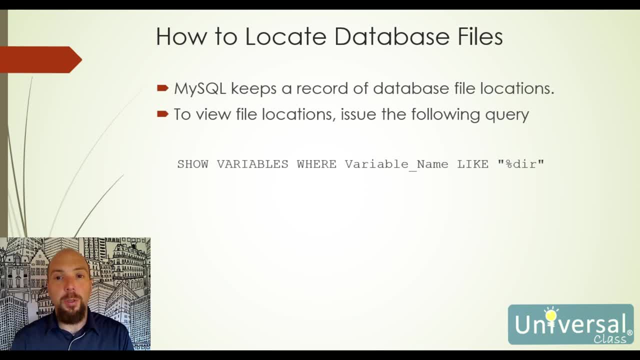 file has the settings for where things are located, what options are turned on and things of that nature. And what it will do is it will take all of the entries that are in that configuration file and loads them in as variables for the system. 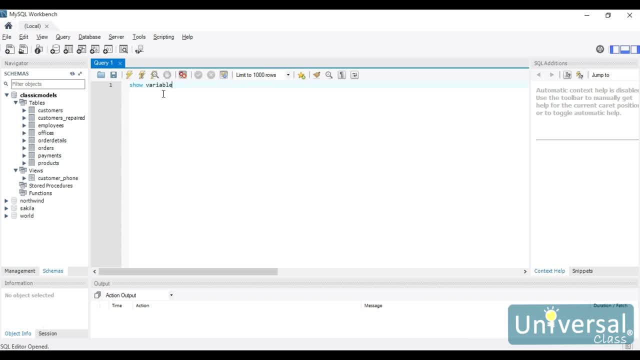 So if I want to know where they're located, I can issue show variables where- and then this is important- you're going to have the case incorrect variable underscore name, And there's a command called like, and what like does is allows us to search for things. 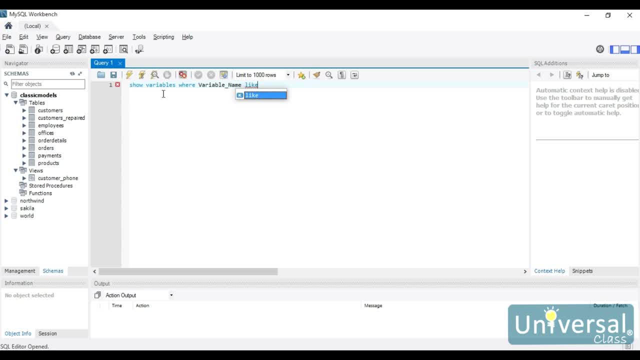 that are similar And one of the variables- I'm sorry, all of the variables- for the directories and in the letters, DIR. So they have beginning characters that may be different, but the last three characters are always DIR. So what I can do is I can tell the system to look for anything that starts with anything. 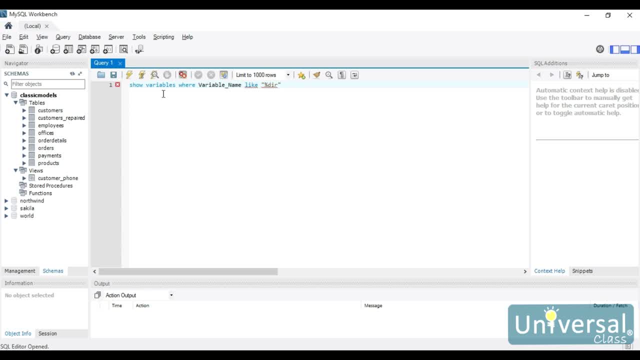 but ends with DIR, and then do this. So what that's going to do is it's going to look for the variable names and it will show us all of the ones that are alike: DIR. So they begin with anything, They can have anything at the beginning, but they have to end with DIR. 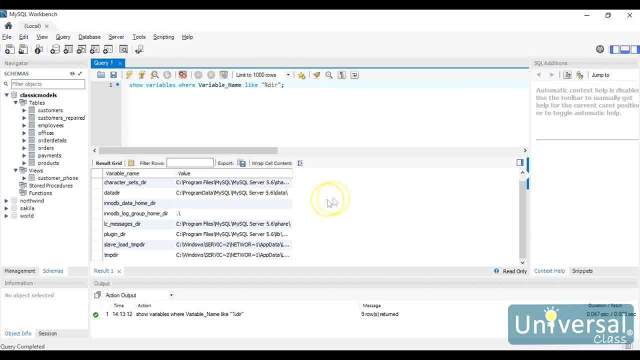 When I issue the command, it will show to us all of the folders where all of our different databases files are located. So, if you notice, he's all end in DIR. So what it's doing is it doesn't matter what it begins with, as long as it ends with DIR. 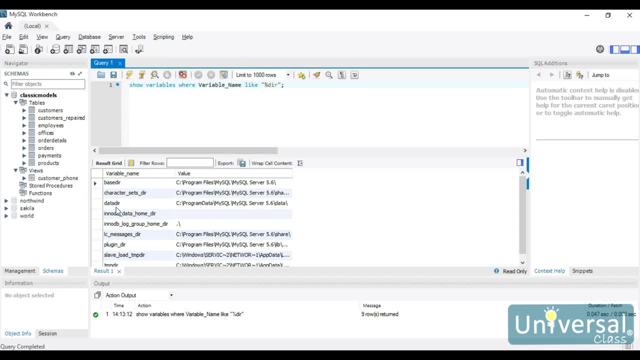 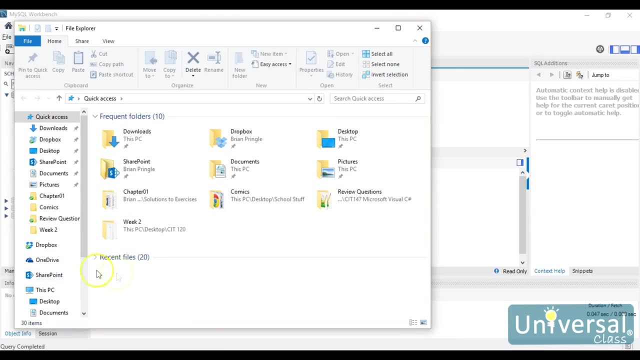 The one in particular that we're looking for is this one right here that says data, dir And notice it's under C colon backslash program data, backslash mysql, mysql server 5.6 data. That's where our actual files are located. So to locate the files, I'm going to open up file explorer. 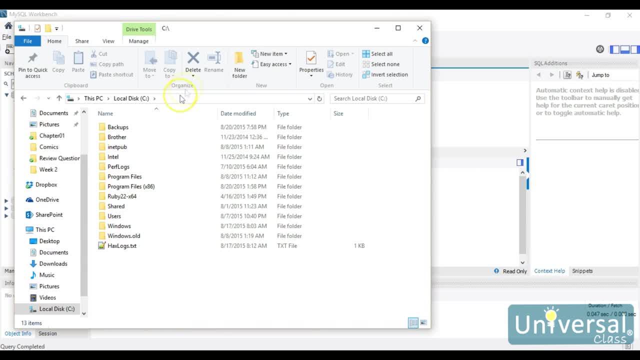 I want to browse to the C drive and you'll notice that program data is not showing in my list. It is a hidden folder, so we actually have to type that in, unless you have hidden files enabled, And so if I scroll down I will see mysql. 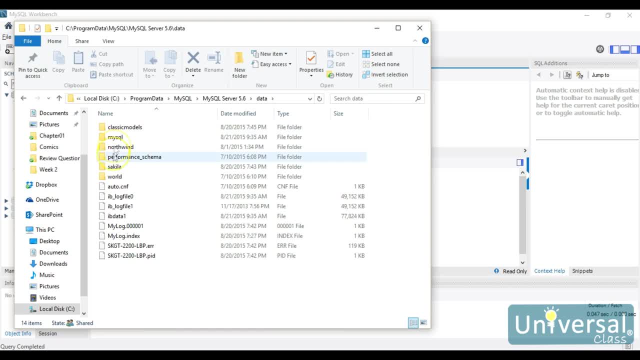 Mysql server 5.6.. And then data. And so this is where our actual database files are stored. You'll notice, each one gets its own folder. So, for example, classic models: we've been using all of the tables, all the forms they're. 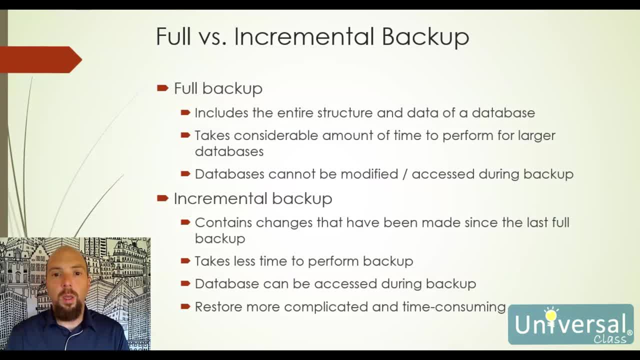 all located right here in this one folder. Once we know where the database files are located, then we can back them up. The problem is, as I stated in a previous lesson, the DBMS has all of these files locked And we actually cannot back them up. All MySQL is running, So the question is: how am I going to back them up? All right, so one of the options is to stop the MySQL services, And when I stop those services, then it will allow me to do a backup of those files. 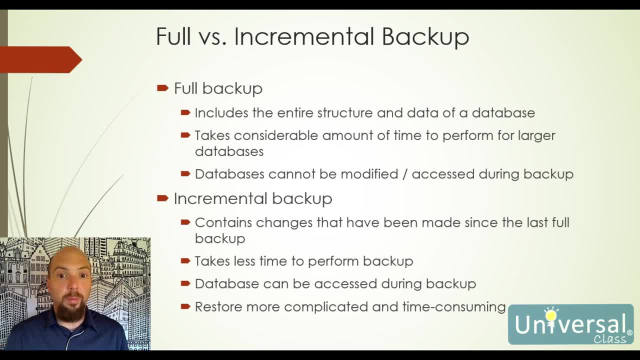 The other option is to use some utilities that are built in. We actually have the ability to do a backup directly in MySQL. it can export all the data. Or the third option is to simply do exports of data. So we have different ways to do backups. 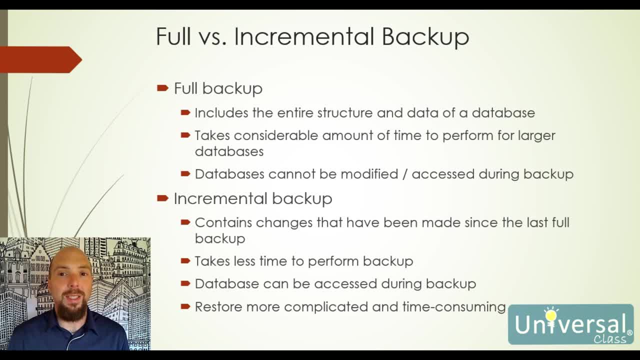 Our first way is to do what's called a full backup. Now, our full backup includes the entire database structure, all the data, all of the tables, all of the roles, everything gets backed up. This takes a considerable amount of time, And the problem is is that the database cannot be accessed during the time when it's actually 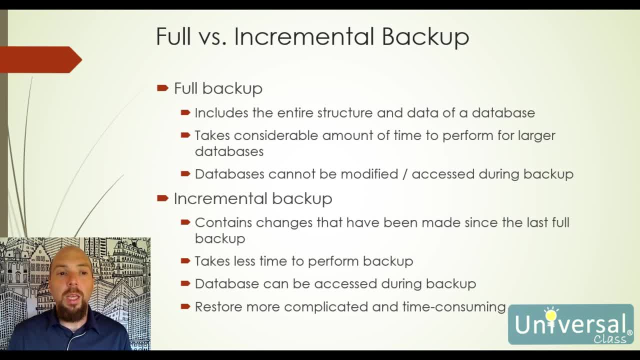 doing the backup because the services actually have to be taken offline. Even if I use the built in backup mechanism, it'll still make the database unavailable to all the users, All right. So another type of backup is called an incremental backup, And what an incremental backup is is that it will only back up the changes that have. 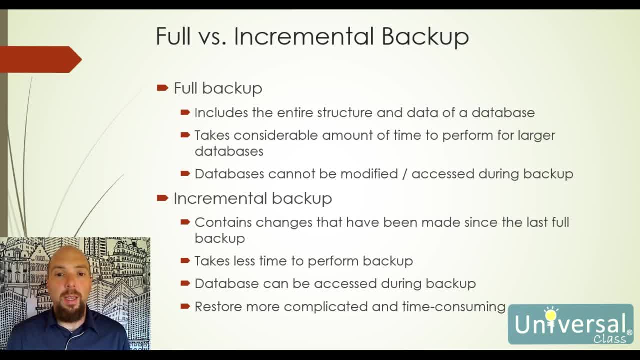 been made since the last full backup. It takes considerably less time to perform these backups and the system can be used while it's doing this type of backup. However, the problem is is when I do a restore of the data, it's actually more difficult. 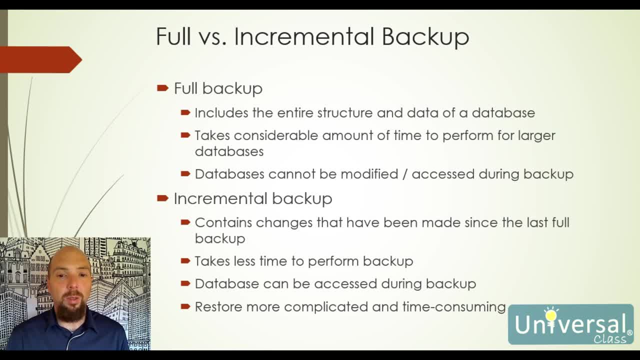 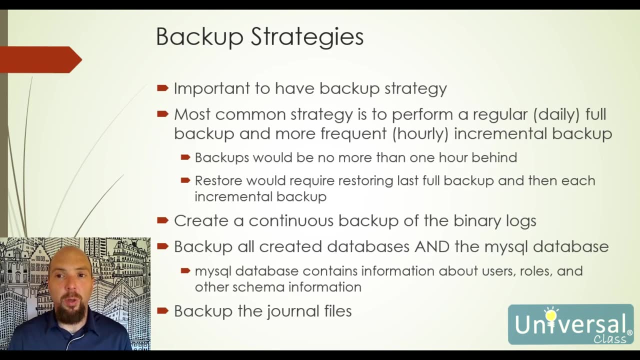 to restore it. So the benefit here is that I can do a full backup, have the entire database backed up and then at regular intervals I can do incremental backups without actually kicking all the users out of the system. So it's very important to have a backup strategy. 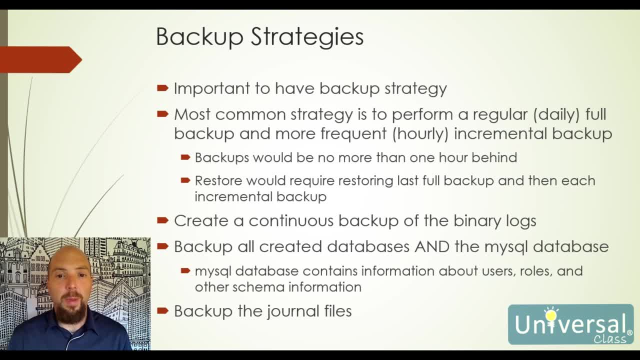 The most common strategy is to use that full daily backup. So typically what you'll see is that a company will do a full backup once a day and then they'll do hourly or even more frequent incremental backups. There are other ways we can do backups. 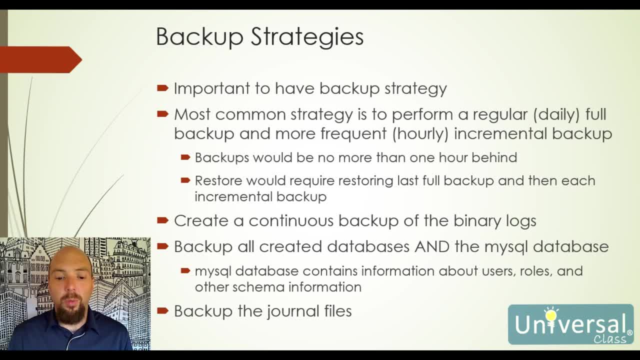 I'll talk to those, or I'll talk to you about those later in this lesson. But the reason for doing this is that if I have the full backup from last night and I have hourly backups and something happens to the server, I'm never more than an hour. 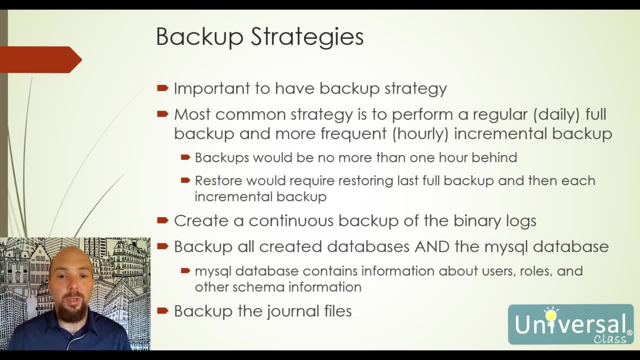 out of backup. So if the last backup was 30 minutes ago, I only lose 30 minutes worth of data. Now there's a way to prevent that from happening, which is there's a thing called the binary log, and the binary log is simply a log that keeps track of all of the changes that have. 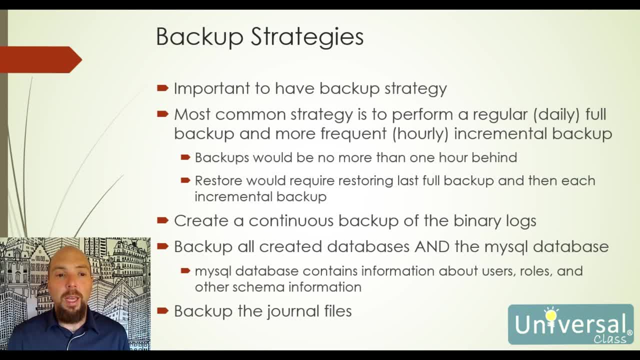 been made to the system. It keeps track of all of the statements, all of the commands, everything that comes through the system. that gets stored. And what we can do is we can do continuous backups of the logs. So what that allows me to do is I do a full backup, say at midnight. I do hourly backups. 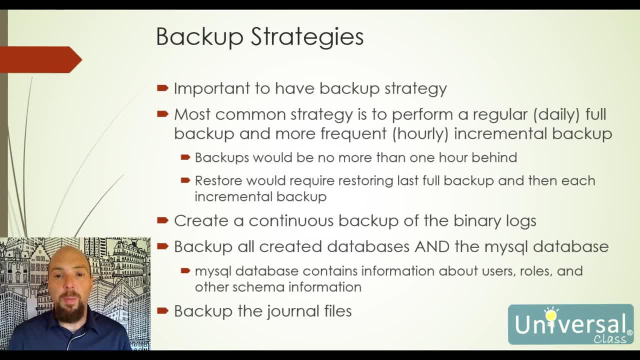 and in between the hourly backups, I backup the log. Well, what that means is that I can restore my full backup, restore all the incremental backups, restore the log And I'm back up and running. There are also these things called the journal files, and we'll explain what those are. 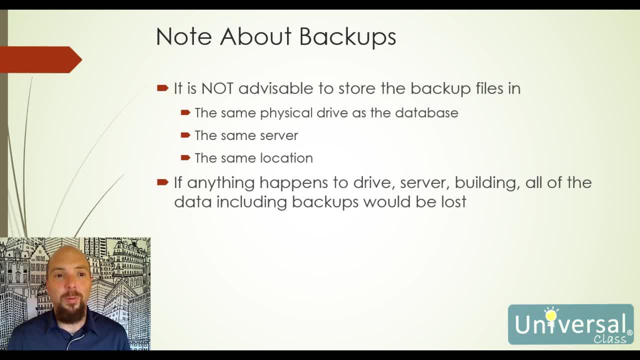 One thing you need to know: it is not advisable to store the backup on the same physical server or the same drive as the actual production server. It's also not advisable to save it in the same location. If you store it on the same server and that server gets fried, it doesn't matter if it. 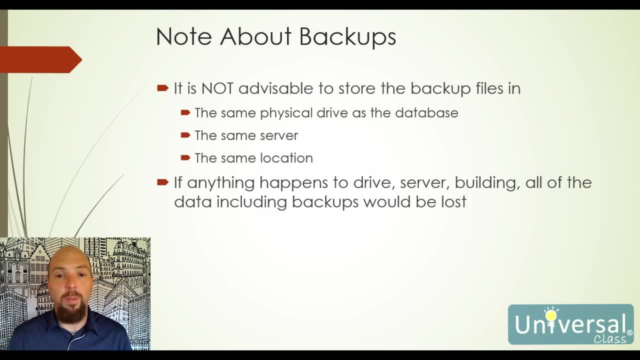 had 10 different hard drives in it. chances are those hard drives are all going to be bad if it takes a big enough power surge. If you save it on the same drive and that drive fails, then the backups are gone. If you save it in the same location and the location catches on fire, gets hit by a tornado. 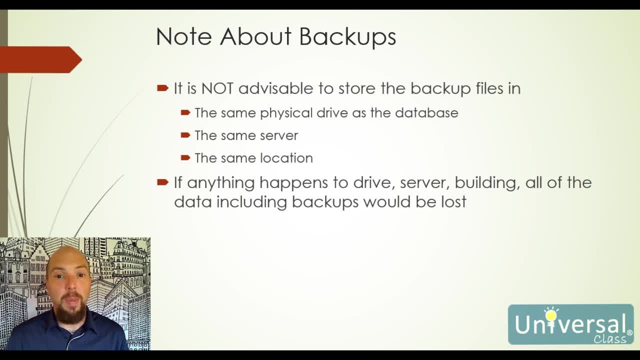 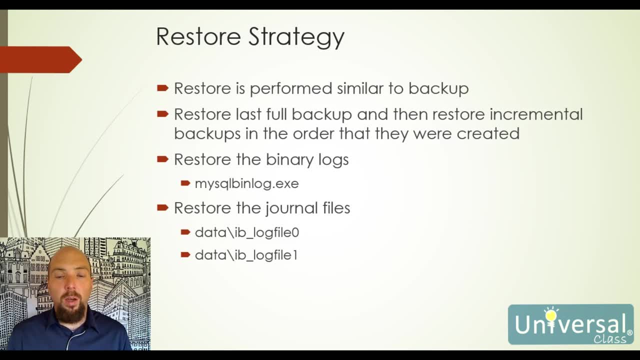 it's all gone. So we want to make sure that the data is backed up to some sort of external media and is stored off site. All right, so I backup my data. I do a full backup at midnight, I do incremental backups every hour and I also backup the log. 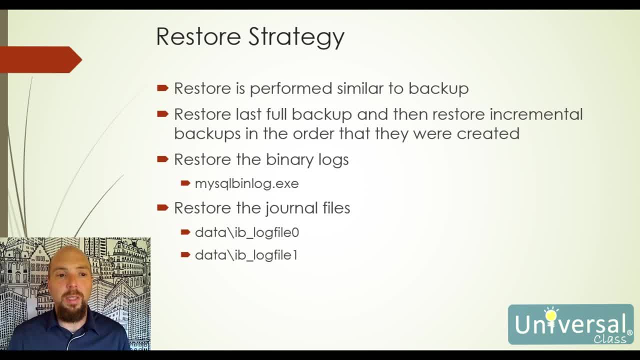 All right. so what I'm doing is I'm keeping all of the data that is in the system, but I'm making it where I'm only doing hourly backups. I only have to do a little bit of backup. I only have to kick the users off at midnight to do that full backup and then throughout. 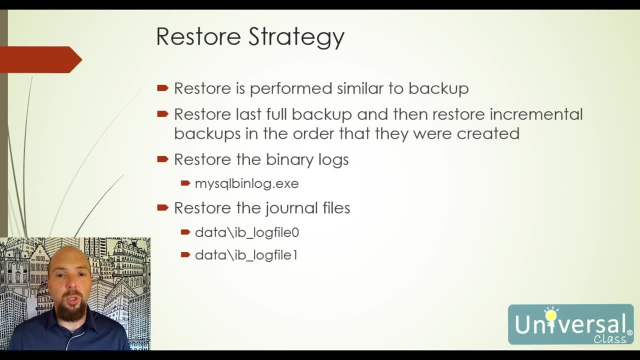 the day. they don't know that we're doing backups. So what I'm going to do is I'm going to restore the backup for midnight, then I will restore each of the hourly incremental backups in order. So I have to do one o'clock, then two o'clock, then three o'clock, and so forth. 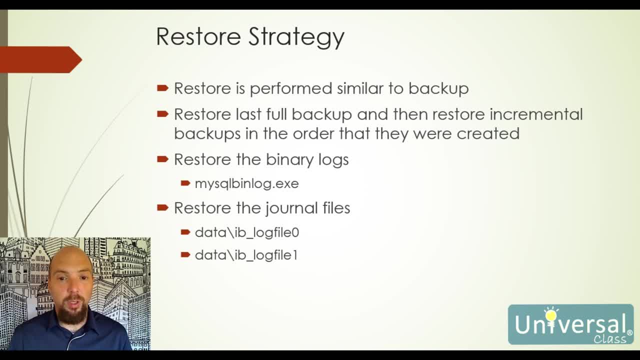 We are going to restore the binary log, which that's the log that keeps all of the statements that have been issued, and then also this thing called the journal files. Now, what happens is MySQL is called a two stage commit, which means that when I actually 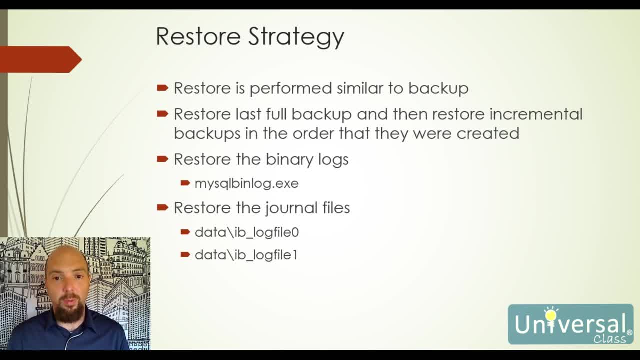 write an entry to the database. so let's say, I want to write a new record, I want to update a record that's already there. then what happens is it gets stored in what's called a journal file, and then it also gets stored in the database. 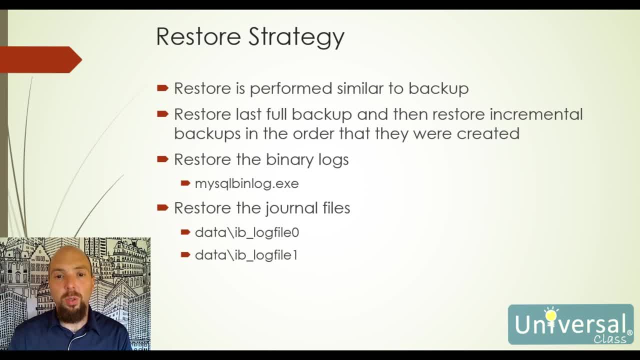 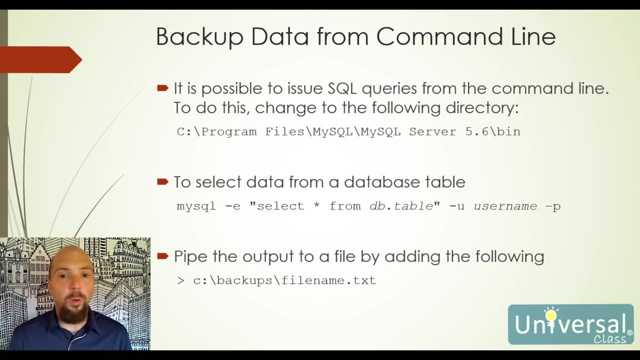 Now it actually is stored in two locations until it has a full commit, and that full commit actually happens during the backup process. So we want to make sure we backup those journal files also. Alright, so I'm going to perform some queries from a command line that will allow me to. 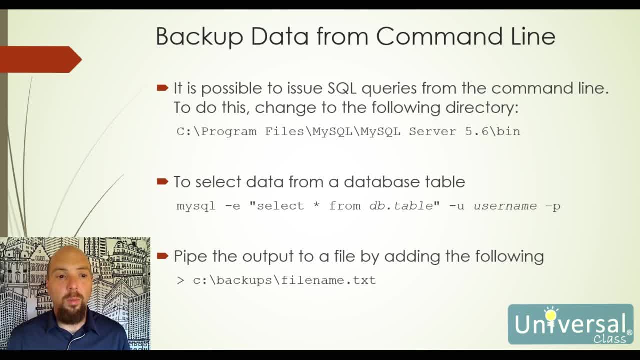 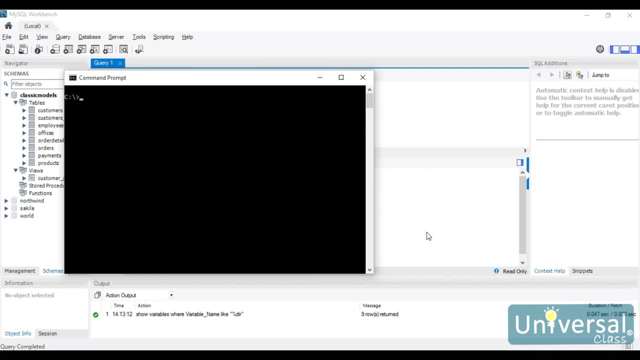 do things like selecting data from a database table, and by doing that we can actually pipe the stuff out to external files. Alright, A command prompt, and on Windows I'm going to do it from the command prompt, on the Mac and in Linux I'm going to do this from a terminal window. 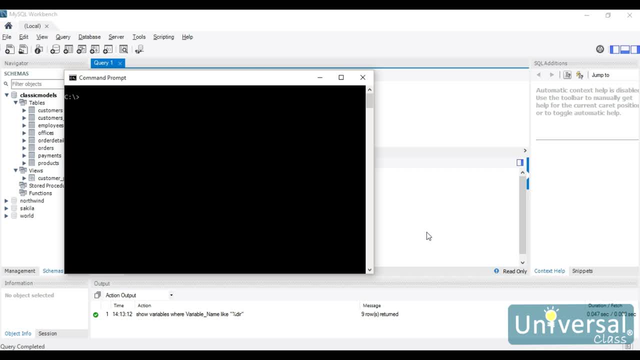 The only difference is going to be how you access the executables. Once you locate the executable, it will be the same commands to actually export the data. So one of the things you need to be aware of is if you have Linux or a Mac, you have. 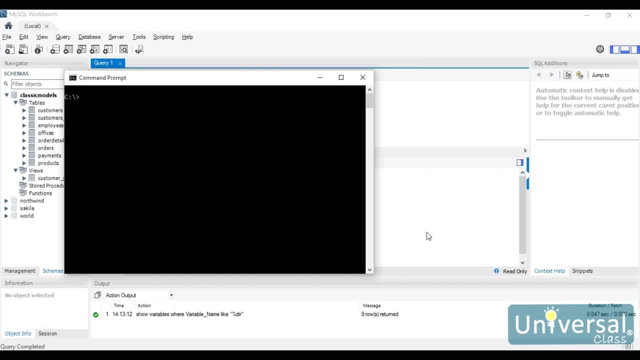 to locate where the data files are. I did show you in a previous video how to find those. So on Windows it's located under Program Files, Under a folder called MySQL, In another folder called MySQL Server 5.6, because that's the version that I have installed. 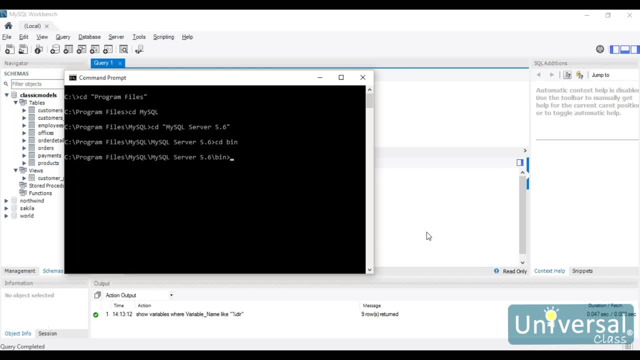 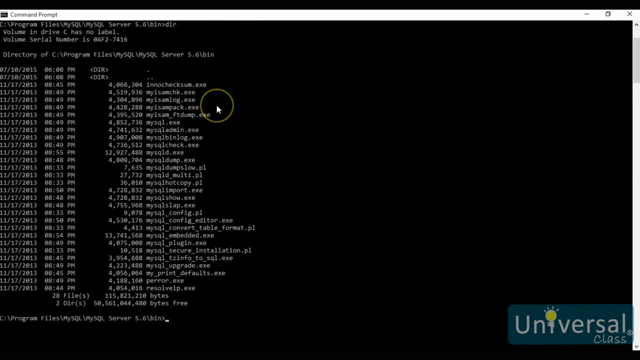 And then in a folder called Bin, And Bin is all of our binary files. So if I look at this, I can see these are all the binary files that we have, And the one that we want to use is the one that just simply says MySQLexe. 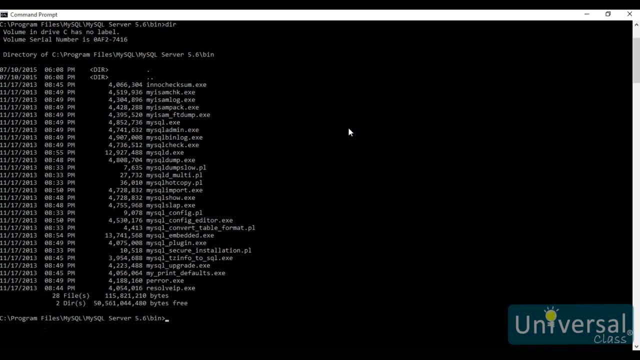 This is our actual command line processor for our database, So I'm going to go ahead and do that. Alright, So this is where all of the statements that we can issue to the system. Okay, so what I want to do is I want to issue a command to the database as if I were sitting. 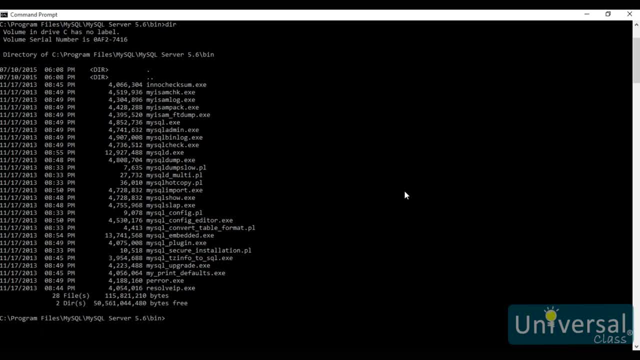 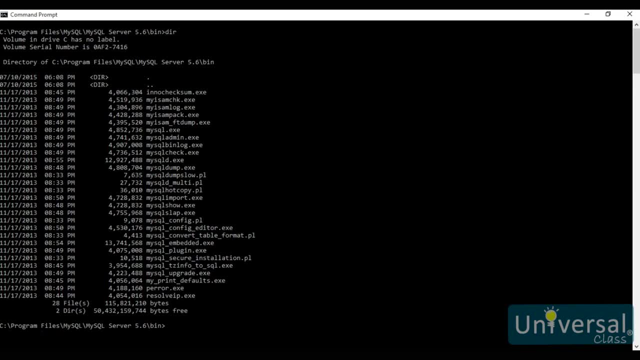 in the actual workbench performing a query. The problem is that I have to authenticate to the system, So when I open up workbench, workbench will ask me for the username and password. Alright, So to do this, I'm going to issue a command stating MySQL, because that's the actual executable. 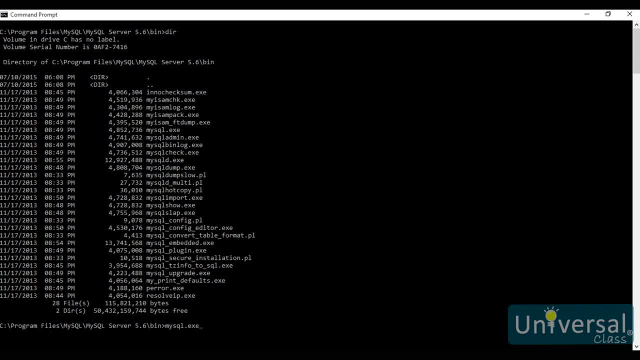 that I want to use, And it's actually MySQLexe. You don't have to type the exe. it will automatically assume that it's an executable And I want to execute something, So I'm going to do minus e for execute. 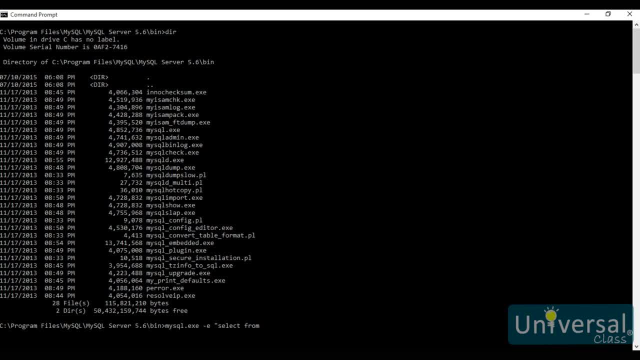 What am I executing? I am executing a select statement. I want to select everything from- sorry, everything from a particular table. Now I haven't told it which database to use, so I'm going to have to do this in the databasetable format. 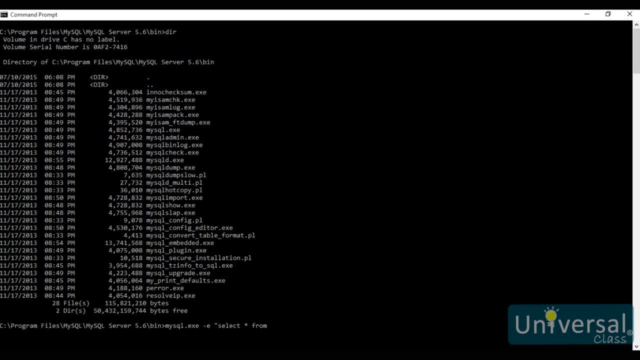 I want to get everything out of the classic modelscustomers table. So I'm going to say classicmodelscustomerstable, And that's what I actually want to perform as my query. So I'm going to select everything from the database called classicmodelscustomerstable. 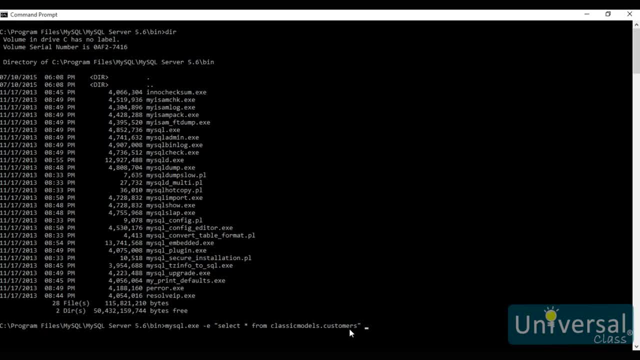 Now I have to authenticate to the system, so I'm going to type minus u and then I type in my username. Now, because this is just for a learning purpose, I am actually using the root account. I hope that in a production environment you don't use root. 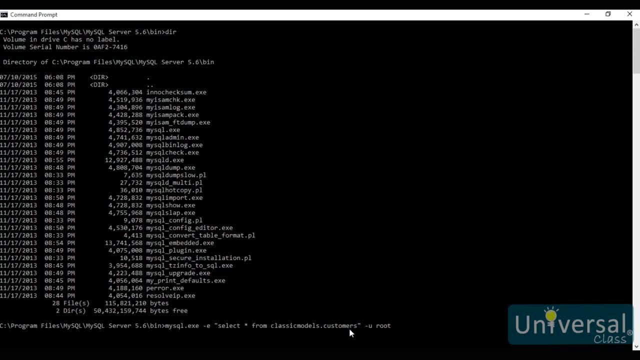 You should be using some separate user account. So I'm going to log in as root and I want to type in my password, but I don't necessarily want it to show my password. So I could type in my password right here and if I type my password then it will automatically. 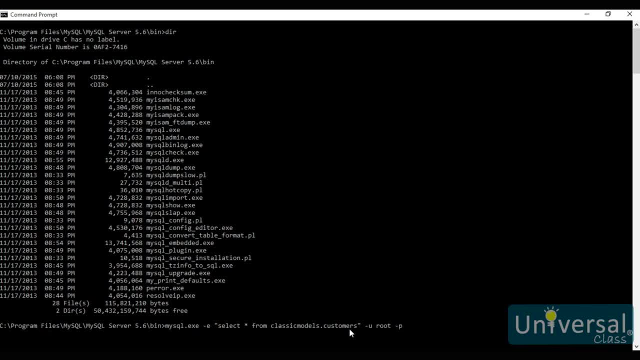 let me in. But if somebody else is standing around while I type my password in, they'll be able to see it because it's written here in clear text. So if I just push enter now, it will prompt me for my password. Type in my password. 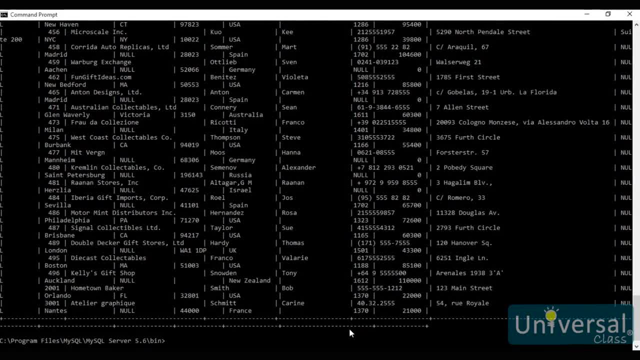 And it executes that query And it actually gives this back to me in the form of a table. So it's a table at the command line. But one of the nice things with the command line is that I can take anything that we have that should be output to the screen, and instead I could pipe that to a file. 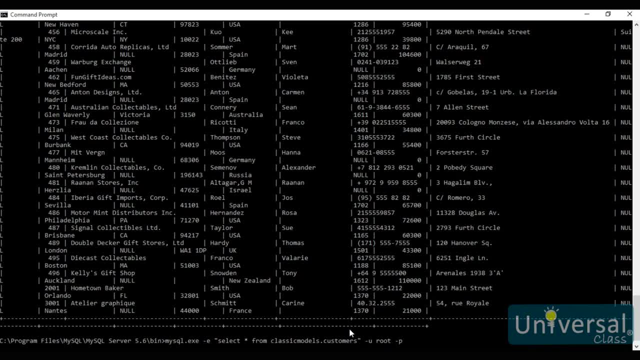 So what I'm going to do is I'm going to issue the exact same command, So I just push the up arrow key and I want to pipe it to a file, so I'm going to output it. I'm not using the greater than sign to some sort of file. 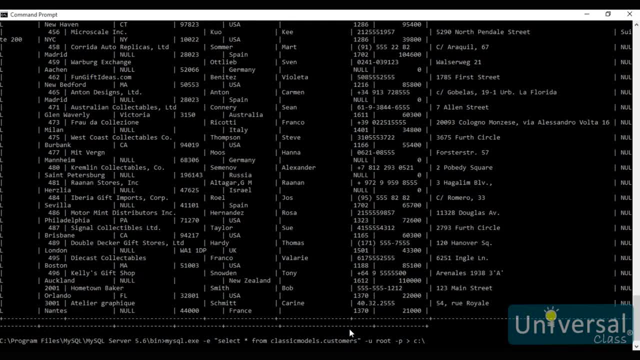 Alright, so what I'm going to do is I'm going to output it to a folder called c, colon back slash backups, and I'm going to give it a name, So I'm going to call it customers dot, txt. And so now what this is going to do is it's going to export all of the stuff that's in. 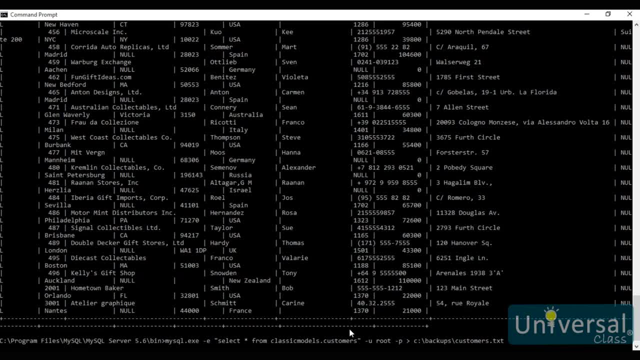 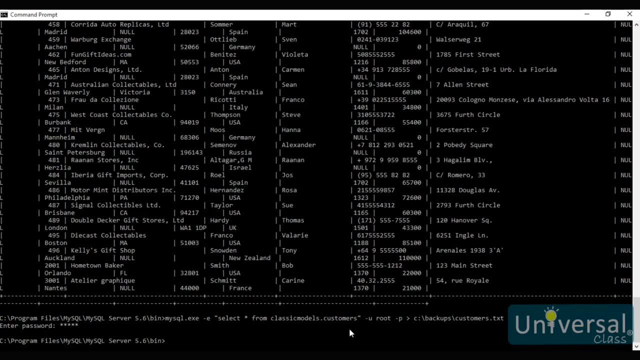 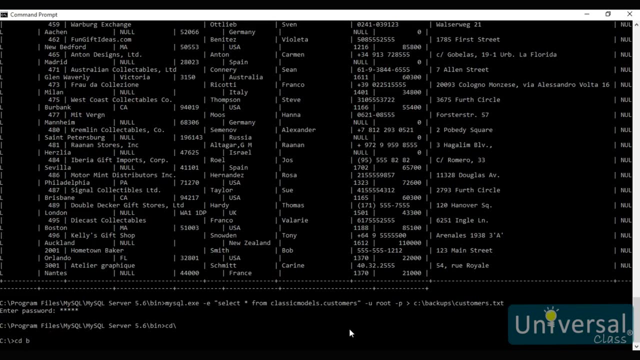 this table and actually put it inside of that text document. for me Now, when I press enter, I won't actually see it do anything, but behind the scenes what it actually just did: It put all of that stuff to that folder. Alright, so I'm going to go back to the root folder. so cd back slash and I want to go to 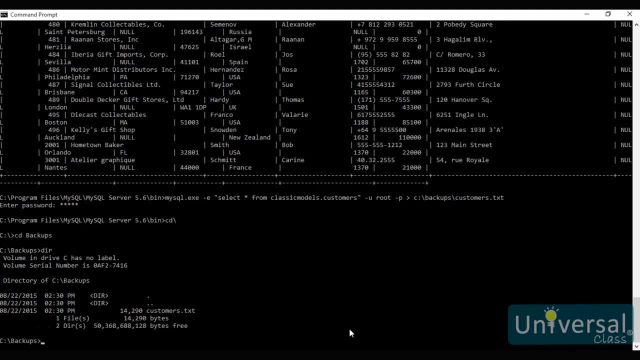 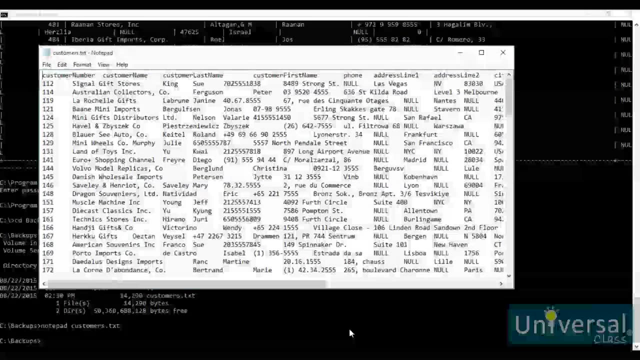 that backups folder And if I do a directory, I will see that I now have a file called customers dot txt. Now if I open this up in notepad or some other program, I can actually access this. So let's do that. Let's look at a notepad. 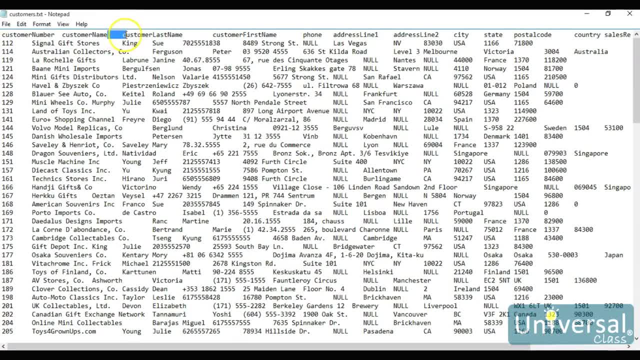 There's our file. Now this is actually going to be- I'm going to call it. It's going to be tab delimited. Notice it's a tab, Which means that I can take this file and I can open it up in excel instead. 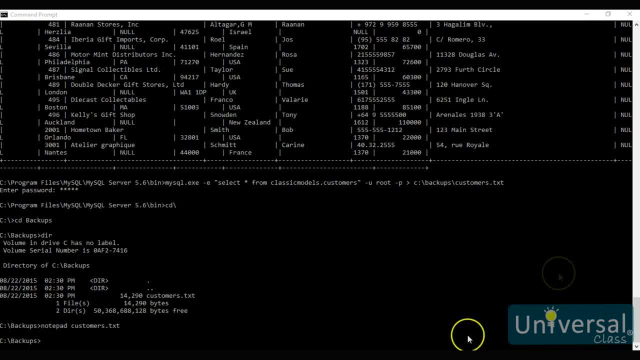 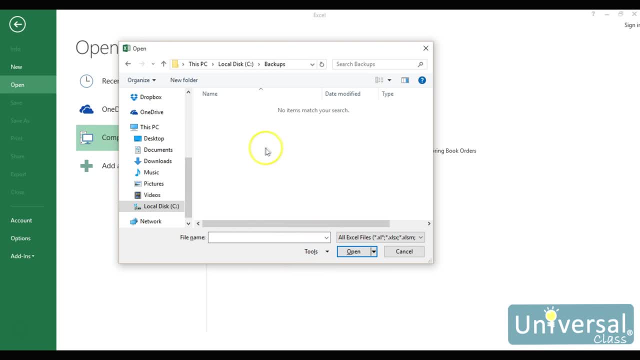 So I'm going to go ahead and open up excel And inside of excel I'm browsing to the backups folder. Now, by default I won't see anything here, but if I change this down here where it says all excel files, I'm going to change this to all files. 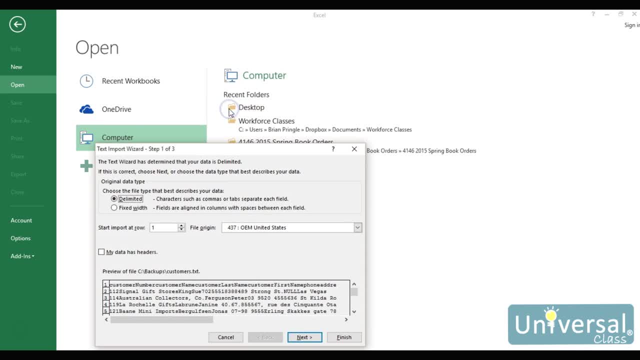 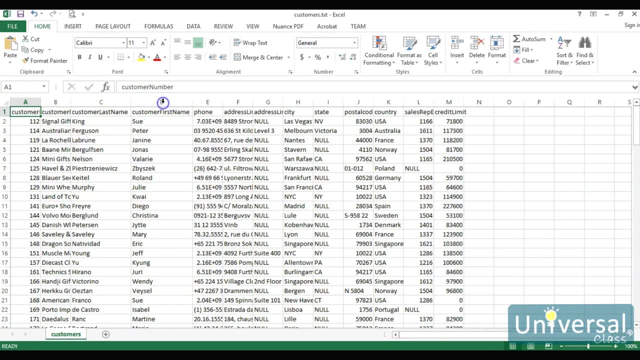 And now I can see my text document is there, And if I open this file It's going to ask me how to import it. I'm just going to go ahead and finish And you will see that you actually do have a table that is accessible. 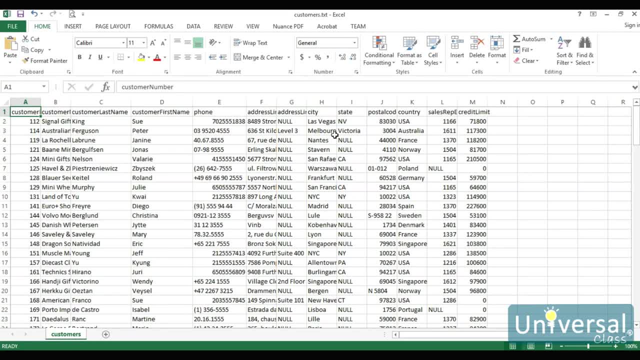 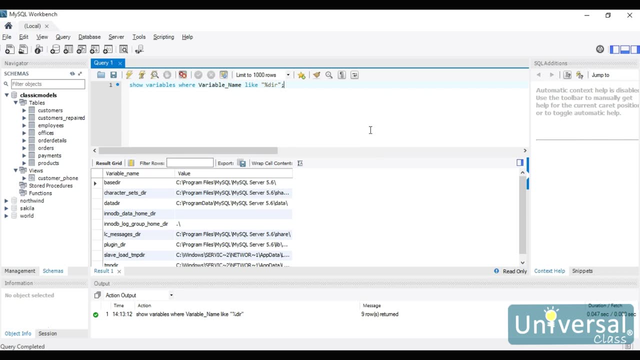 It's just a tab delimited table. So I now have something that is exported out into a tab delimited file that I can use as a backup of that table, And I can also use that to get it into another system. My other option is to do what's called a dump. 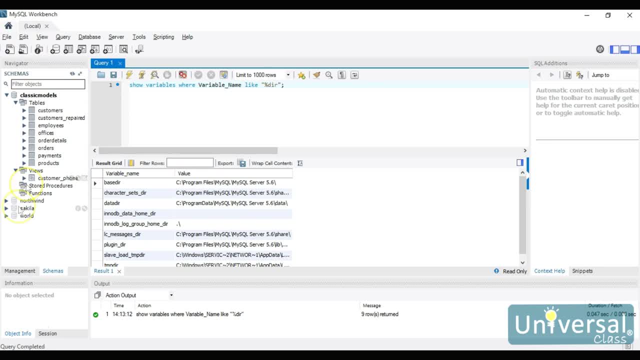 And I'm going to do a dump from the workbench. And the way that you do it Is: I'm logged in and on the left side here you'll see management, And when you go into management, what I can do is: I can. I can simply go to data export. 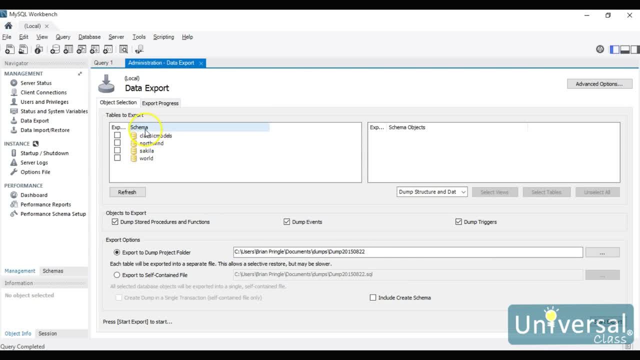 over here And when I export the data, I have my database, my databases or my schemas listed here And I want to export everything that's in classic models. Now, if I click on it, I could export just individual tables, but I want to do the whole thing. 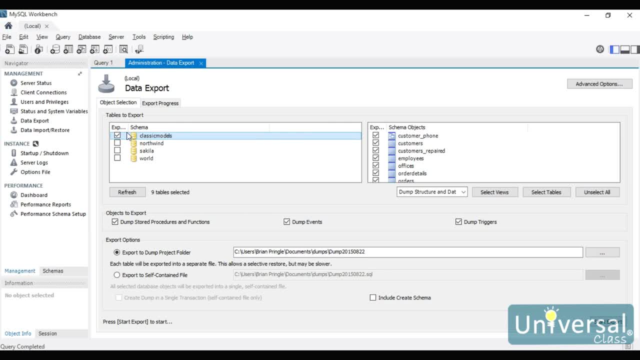 Alright. So what I'm going to do Is I'm going to do what's called a dump, And what a dump will do is just take everything that we currently have And it will output it all to the hard drive as files. 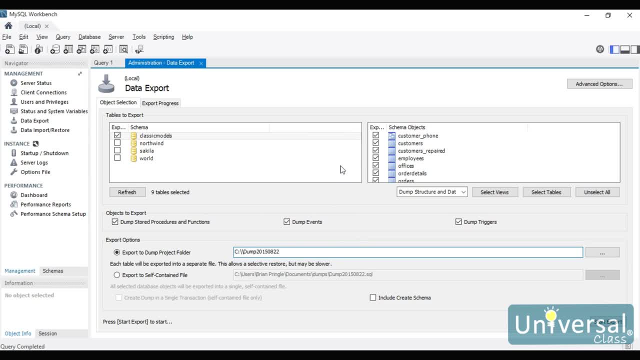 So, instead of having this in my users folder, I'm going to put this in backups And I'm going to leave it as this dump and, if you notice, by default it will be the year, month and date, So that way you can identify when the dump was created. 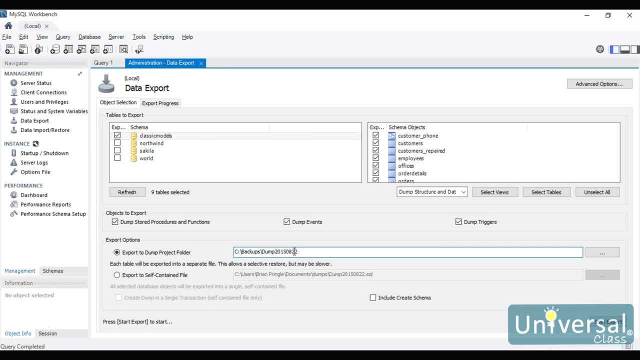 If you're going to do more than one dump a day, you want to change this to something else? Okay, So here are the things that we have selected. We have the schema selected. We have all of the tables selected. I'm going to dump stored procedures and functions. 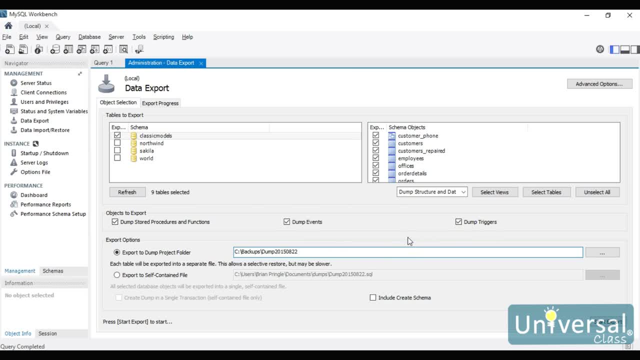 We're going to dump events, dump triggers, So essentially we want to dump everything. We want to make it where I can export everything from the system, so that way I can recreate this on any other system or even back on this one if something happens to it. 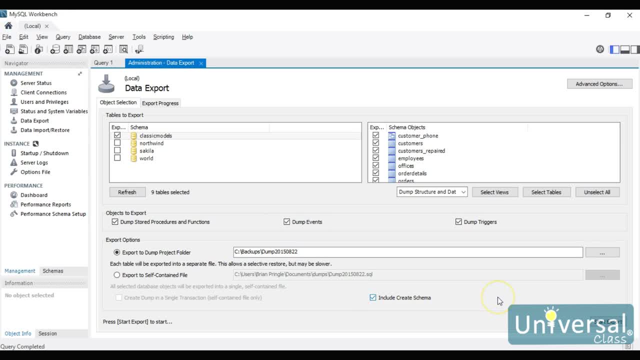 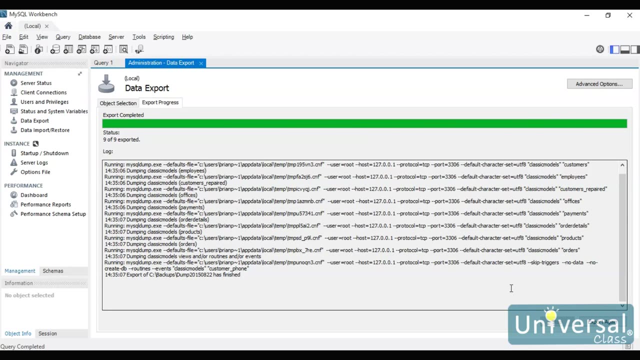 So I also want to include this. one says include create schema, And what this will do is it will actually put the command into the exported files, that it will automatically rebuild the database and rebuild all of the tables. Okay, All right, So I'm going to go ahead and start the export. 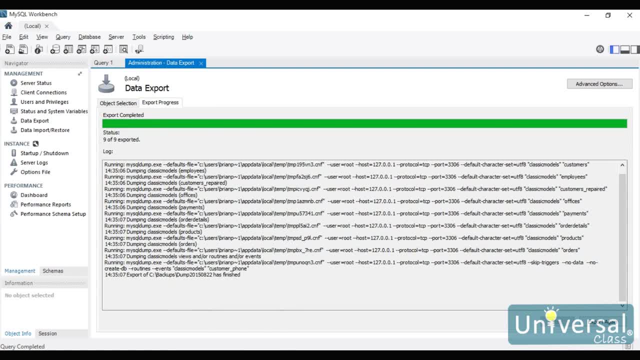 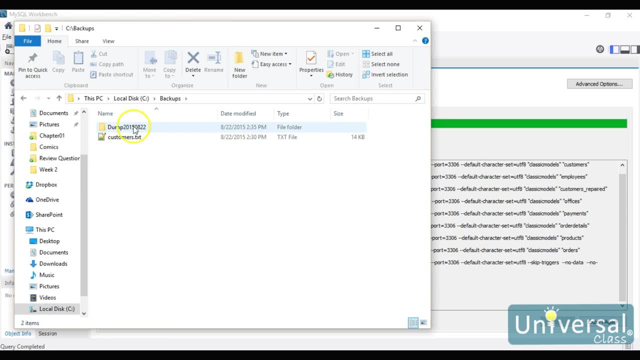 It ran and it is completed, All right. So what I want to do is I want to go back to the C drive, to our backups folder, and I now have a dump folder, and inside of our dump folder are our SQL files for each of the tables. 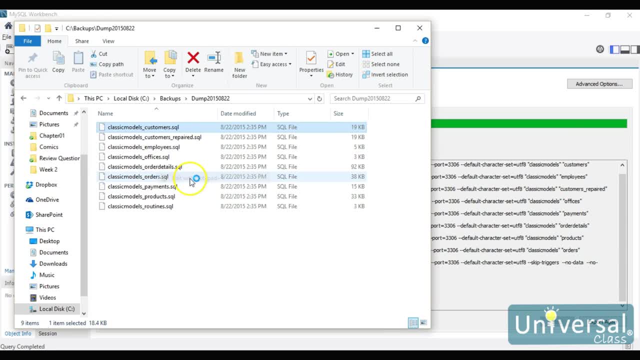 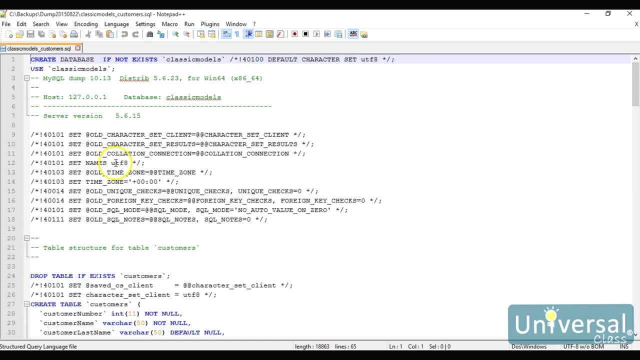 that are there. So if I look at this customers table, I'm going to open it with a notepad, plus, plus, Okay. And what it actually does is it creates all of the statements that are required to recreate it. So create the database if it doesn't exist. 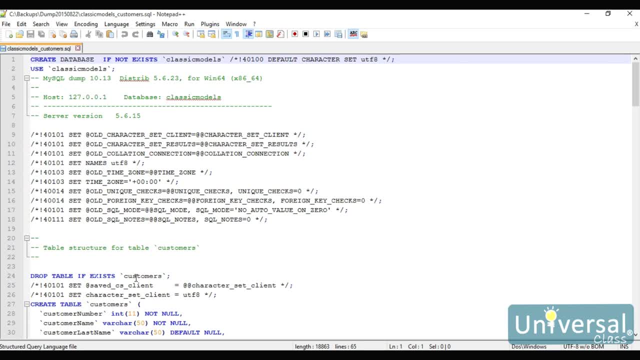 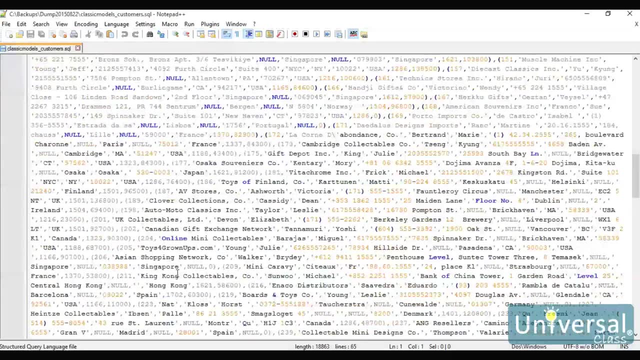 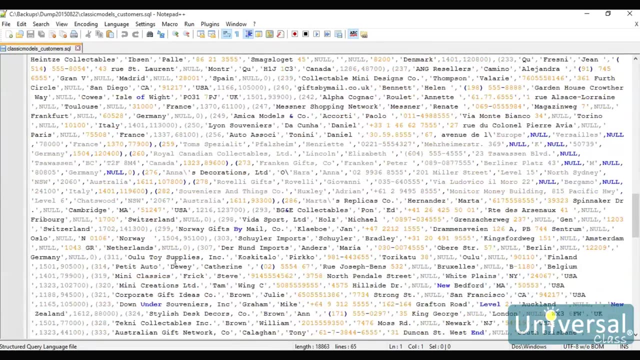 Then also drop all of the tables. that way, if we have a database table that gets corrupted, it will dump the entire table and it will rebuild it from this last set. So this is an actual full backup of that database. The only problem is, while this is running, none of the users could be in. 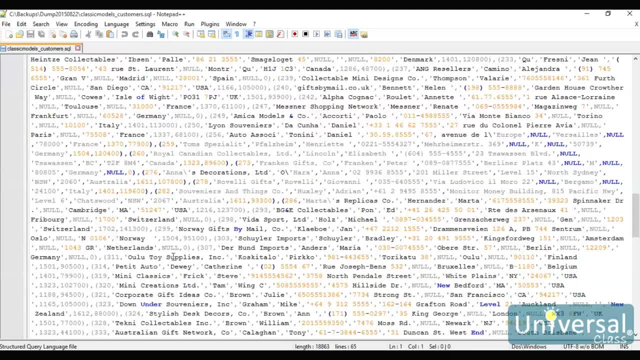 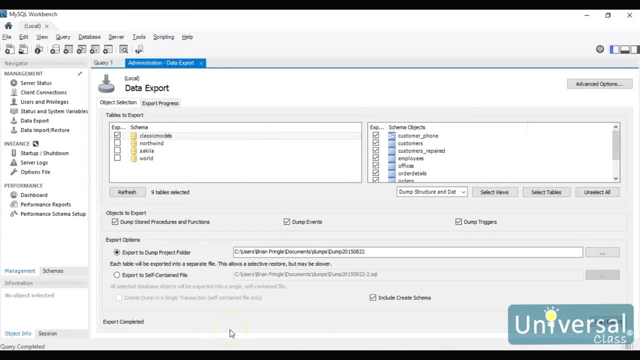 So just keep that in mind. When we do a full backup like this, the entire system. no users can be in it. We would have gotten an error if there were people in it. I do also have another option for doing backups: Instead of backing up as individual files within a folder, I could back this whole thing. 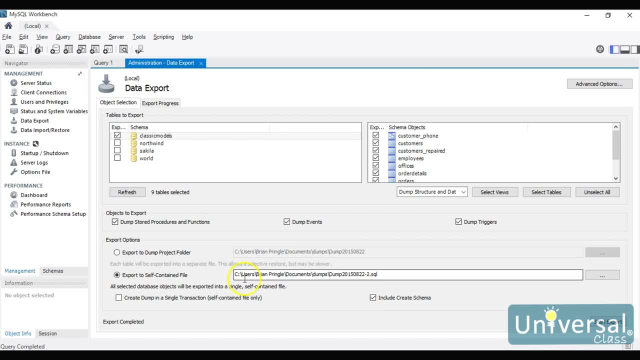 up as one self-contained file, And so what I'm going to do is, once again, I'm going to change the location to our backups folder And the options here are going to be the same. So we're going to include the schema Dump, everything. 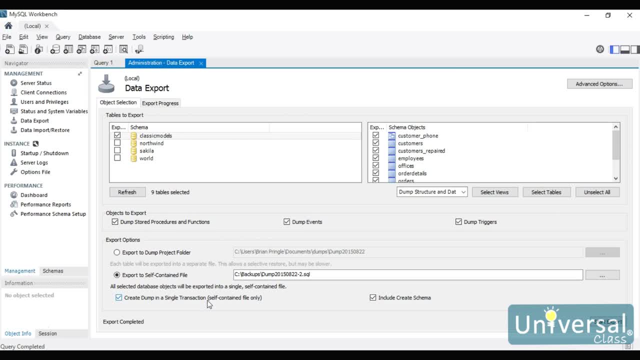 But I'm also going to create the dump in a single transaction. This will make it all one self-contained file to rebuild the entire database. The negative to doing this is going to be that if I want to restore just one database table, I can't do it. 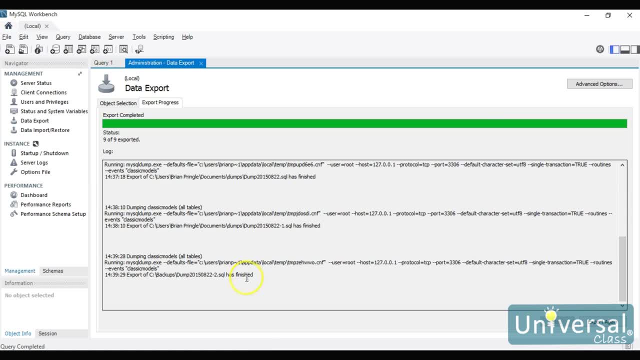 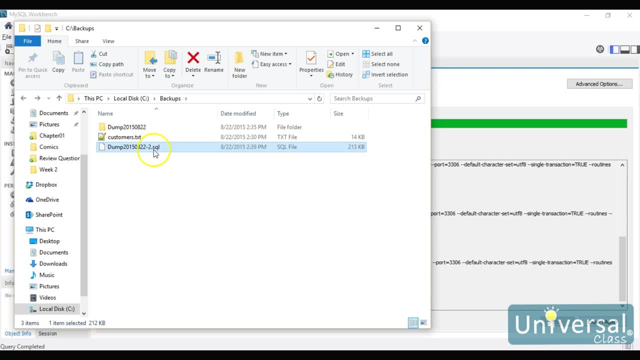 I have to restore the whole thing. So I'm going to start this. We'll let it run. It says it finished. So if I go look at my backups folder, I now have a file here. It's a sql. If I open it with Notepad++, same thing. 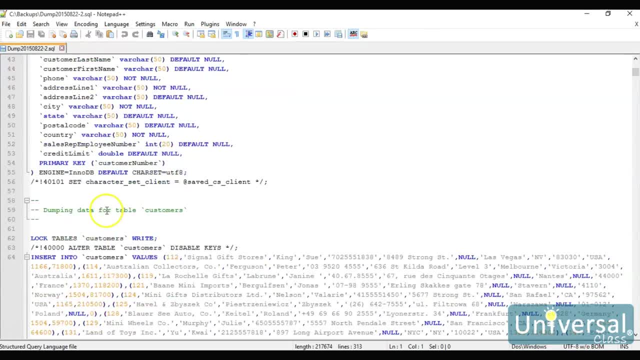 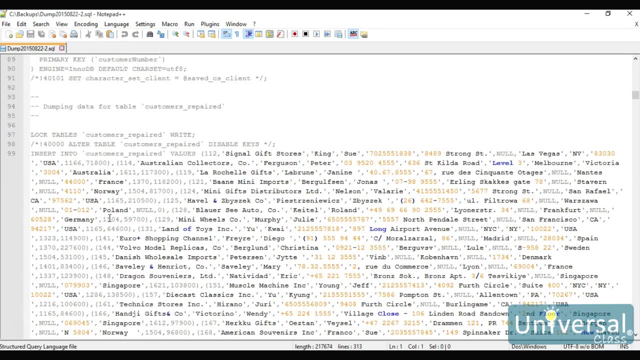 We have the full structure of the database And what it's actually done is given all of the statements required to rebuild all the stuff that is in the different tables. Now, if you're on a Linux machine or Unix or a Mac or something like that and you don't, 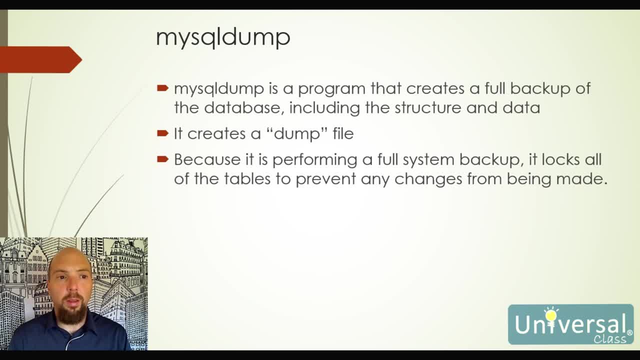 have the workbench installed. you can do this from a command line. There's a utility called mysqldump And what it will do is it will create the same dump files just from the command line. The problem is It does a full system backup and it locks all of the tables, which means nobody can make. 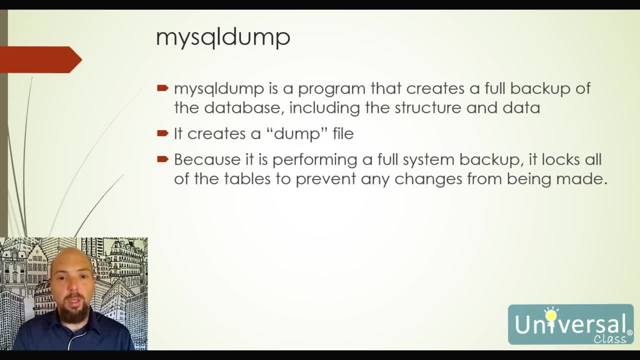 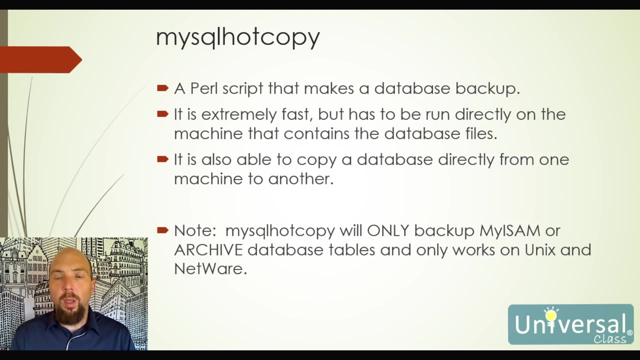 any changes while it's being performed. Now, the database that I'm using is rather small and it did the backup fairly quickly. If you have a very large database table or a large amount of database tables, it will take considerably longer to do the backup. 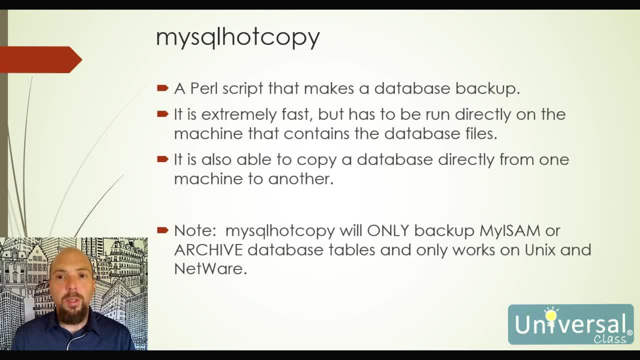 There's also a program called mysqlhotcopy. Now, this is going to be a Perl script that makes a database backup, And You can use this with the myisam or archive database tables, and it only works on either Unix or NetWare. 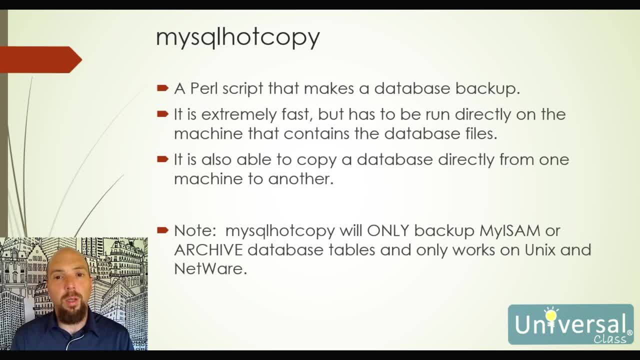 But if you're using one of the older database formats and you're using Unix or NetWare, then you can actually use this utility. It is extremely fast at actually making a backup of the whole database. It has to be run directly on the machine. 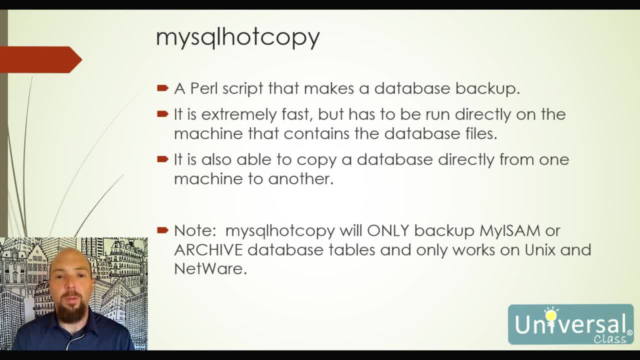 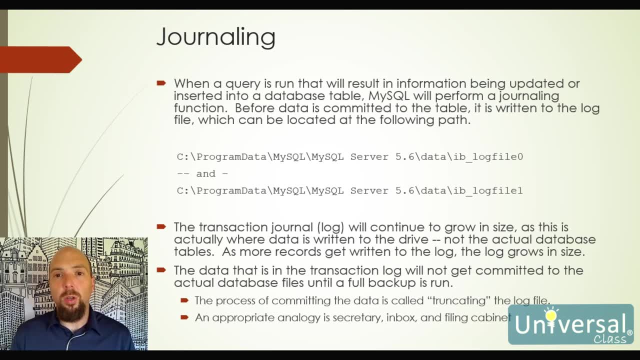 But the benefit of this program is that it actually will allow you to copy the entire database from one system to another fairly quickly. Alright, so something that you need to understand is this process called journaling. What happens is when you actually perform a query and you update or insert information. 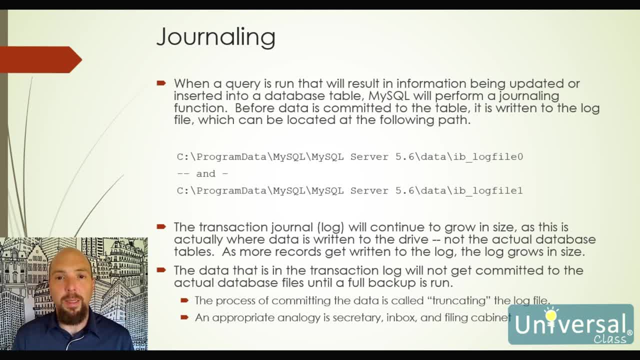 into a database table. it actually does not become part of the database itself. It becomes part of what's called a journal file or a log file, And in Windows they are located at the C program data, mysql, mysql server 5.6 data and then 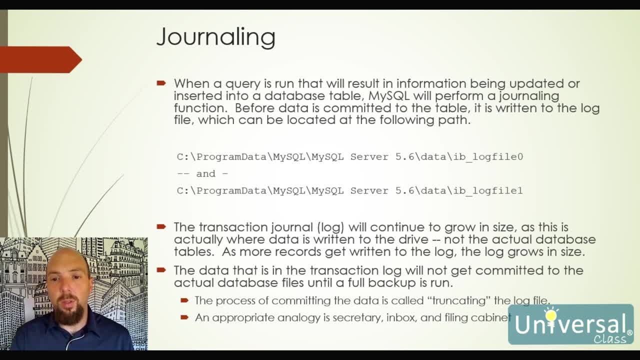 it's called iblogfile0 and logfile1.. And Those are the two files that are typically used. If you have a large environment, you can expand those, but this is the typical version. So what happens is I want to update something in the database. 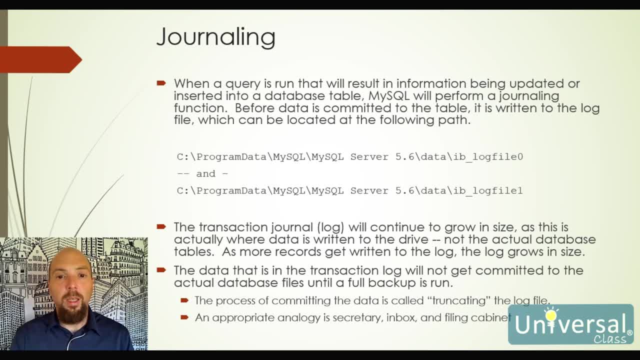 I want to change somebody's telephone number or their balance or something like that, I can't directly edit it in the database, and that's there as a protection, Because if I were to update something into the database itself and something happens to the database before the next incremental backup occurs, 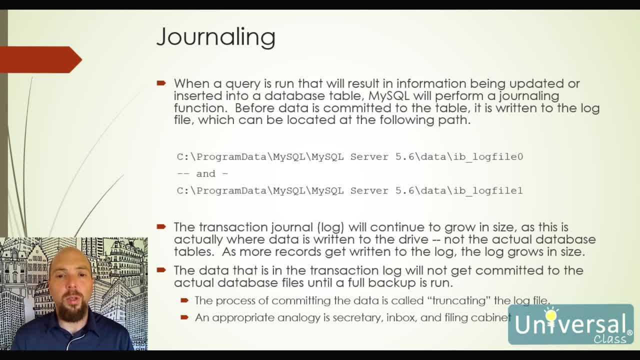 My transaction gets lost. So the way the system works is it will write my query to the log file and then it will also write it to the database table. after it's successfully written to the log, All right. But what happens is it doesn't fully commit the data until we run a backup. 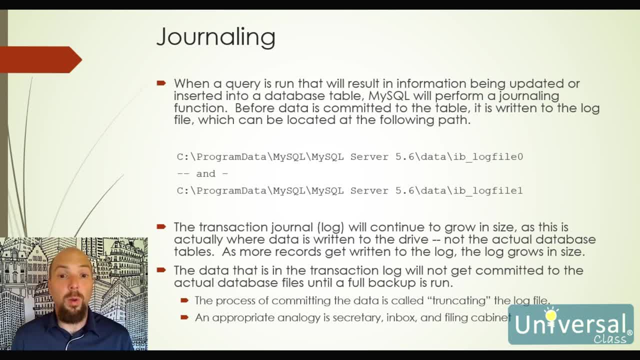 And so what will happen is these log files will continue to grow and grow and grow in size until the until the backup occurs. All right, So what happens is I write my update to the log. It got written to the log Now it writes it to the database and the log file just keeps growing. 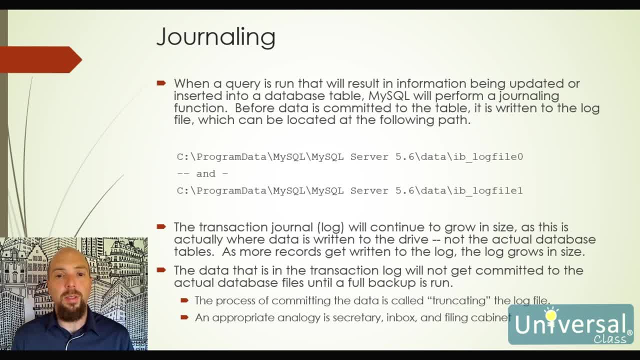 So what happens is you'll have users that start complaining that the system is running slow, especially if you don't do regular backups, Because the log file runs. I'm sorry, the log file will grow in size until the database actually gets backed up. All right, 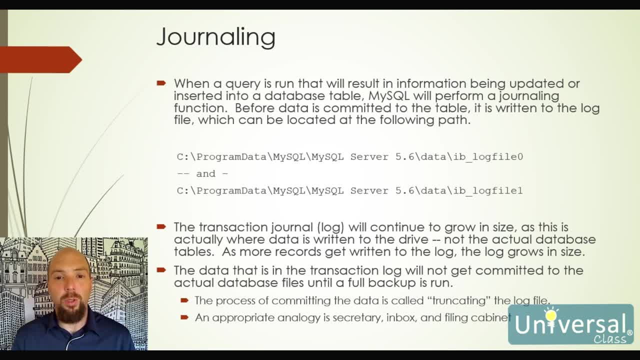 So what happens is during the backup, there's this process called truncation. which truncation will do is it'll take all the stuff that's in the log and it will ensure that it's committed to the database and then it then it actually will delete the data from the log. 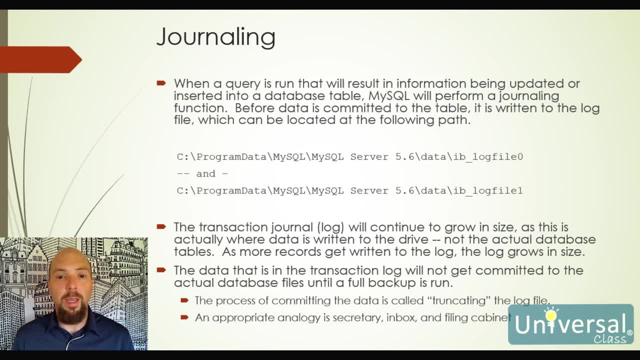 All right. So an appropriate analogy for this would be like a secretary that has an inbox and his or her desk and also has a filing cabinet. Now the secretary. anytime anybody wants to provide updates to whatever is in the filing cabinet, the secretary will not open the filing cabinet. 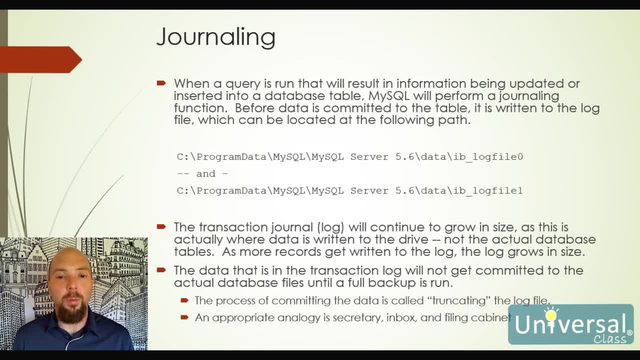 What the secretary will do is: the secretary will hand a piece of paper to the person asking them to write the updated information on the piece of paper. Then what will happen is the piece of paper gets put on the top of the stack, that's in the inbox. 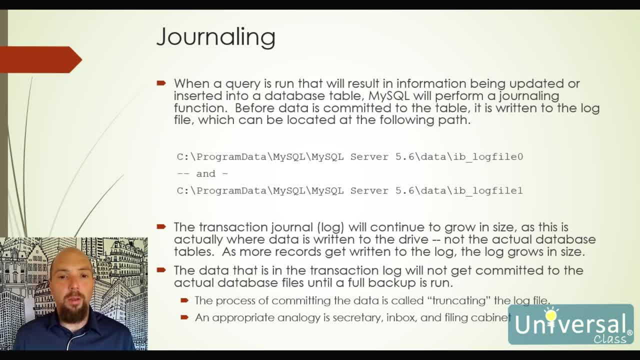 All right. So what happens is: let's say I have, I have a customer that has a balance right now of one hundred dollars. Then what will happen is if the customer comes in and wants to, wants to deposit two hundred dollars in the account, They start with a hundred dollars. 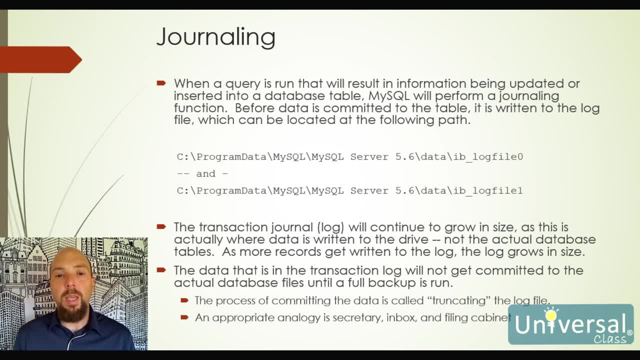 They add two hundred dollars. They should have three hundred dollars in their account, But what actually happens is the hundred dollars stays in the filing cabinet. There's a piece of paper in there with the customer's balance and that stays in the filing cabinet. 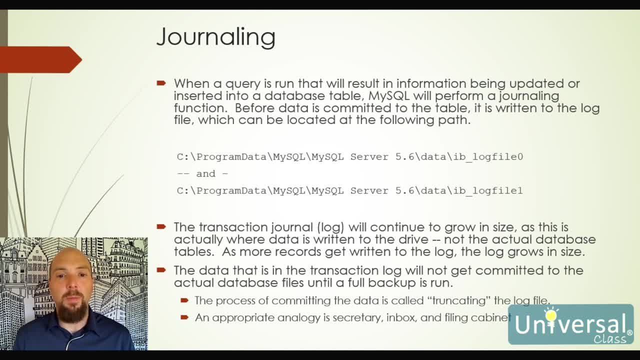 And then on the piece of paper that the person writes down and sticks in the inbox, that one says to add two hundred dollars to it. The customer comes back later in the same day, withdraws fifty dollars. So another piece of paper gets written that says: subtract fifty dollars from it. 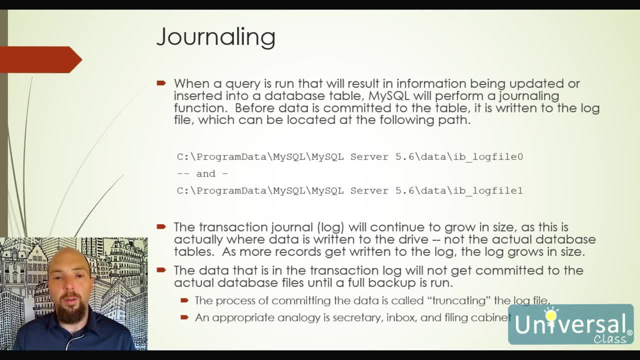 So what will happen is it's It's actually keeping track of what the balance was at the time that that piece of paper was put into the system. So if I want to know what the current balance is for that person, then what I have to do 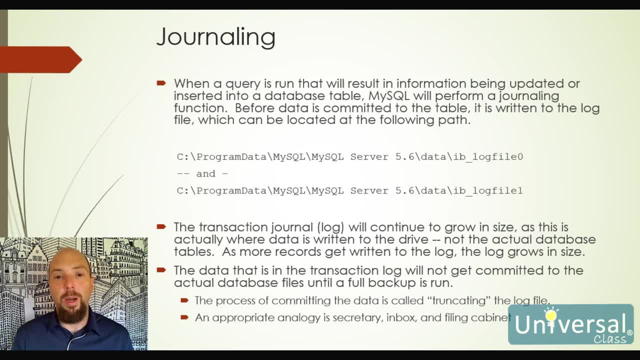 is. I have to go check the filing cabinet to see if they have a record in there. So I look at the filing cabinet. filing cabinet still says they have a hundred dollars. Then I start in the stack of papers at the bottom and go through one piece of paper at. 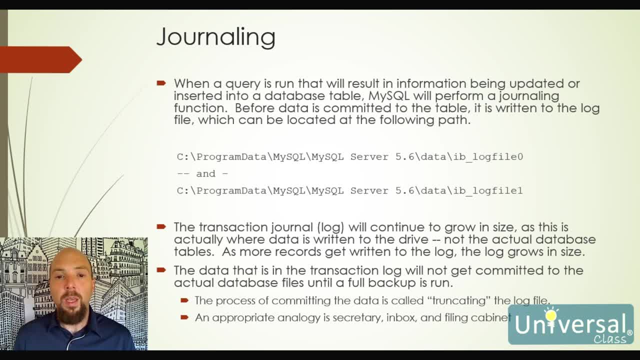 a time until I find a piece of paper that has something to do with that customer, And then I can look at their balance on that one. Oh OK, it's not a hundred dollars, it's three hundred dollars. Then I have to keep going through the stack until I find the next piece of paper that 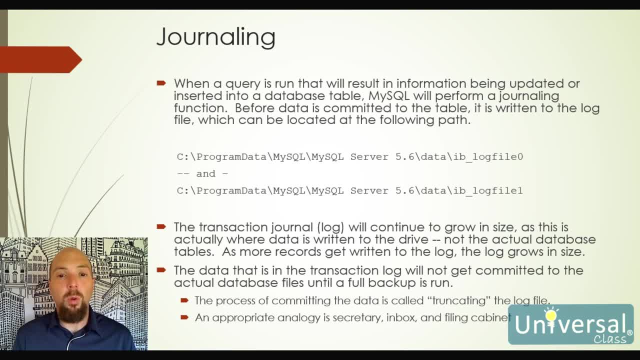 says: oh no, it's not three hundred dollars, it's two hundred fifty dollars. Then I have to keep going all the way to the end of the stack until I run out of pieces of paper to realize that I don't have any more transactions for that person. 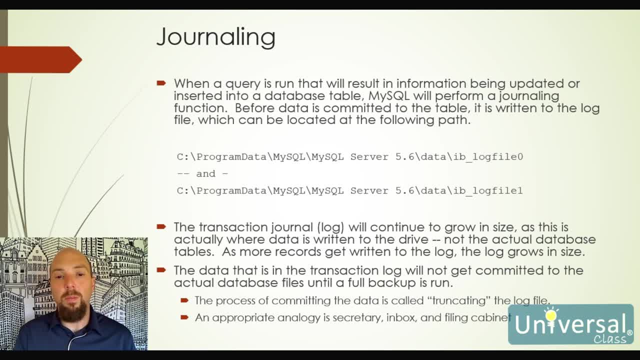 So what happens is the secretary is not going to commit the stuff to the filing cabinet until the end of the day. That's our backup process. So when we do a backup, we take all the pieces of paper Out of the filing cabinet- I'm sorry, out of the inbox- and stick them into the filing cabinet. 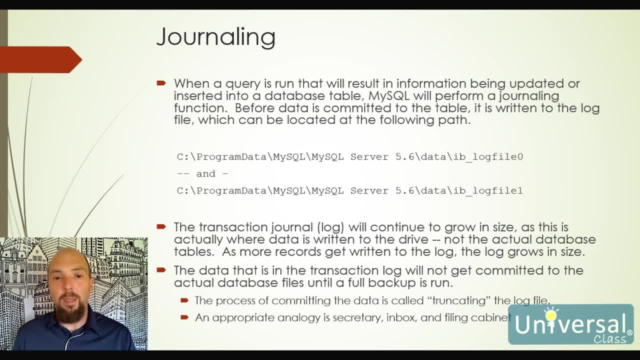 and now they're committed and now the inbox is empty. So the inbox is like our log file. The filing cabinet is like our actual data database tables. So if I want to update something I have to put it in the inbox first. Then it can be put into the actual database. 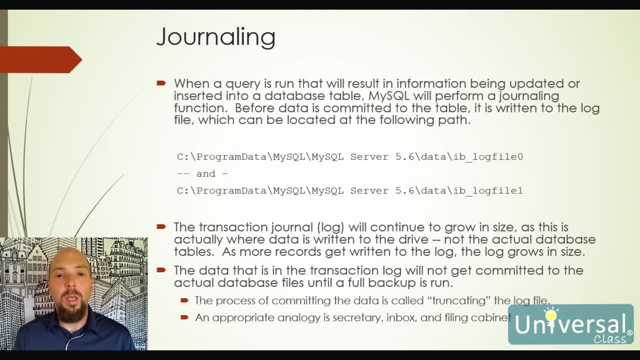 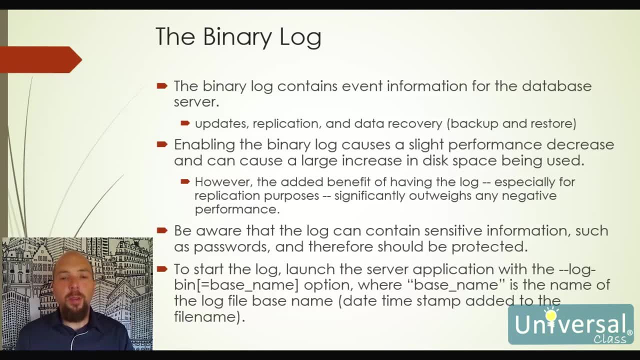 But the problem is is the size of the inbox is going to keep growing until it all gets committed to the filing cabinet, and that occurs during the backup process. There is another important file that we need to keep track of, which is called the binary log. 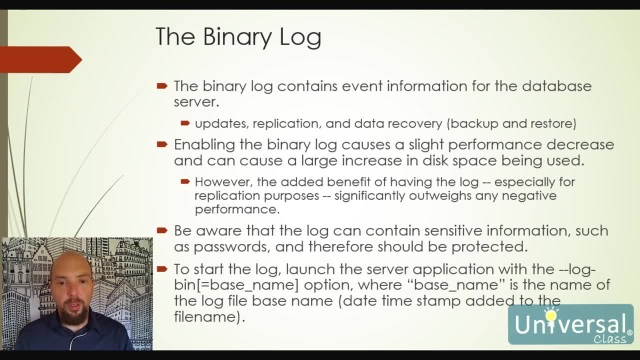 By default, this is not turned on. We'll actually have to turn it on for some of the capabilities that we want to add later in this lesson. The binary log is responsible for keeping track of all of the updates, all of the replication, data recovery, backups, restores everything. 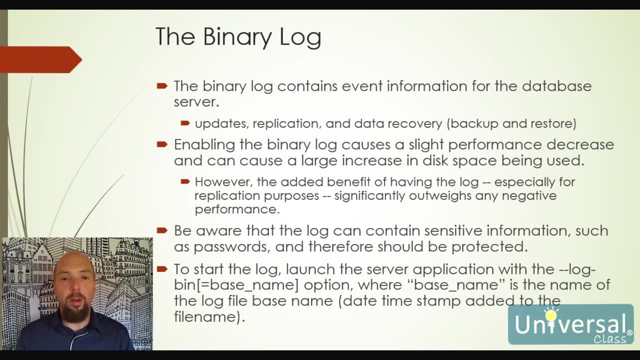 So everything that happens to the system gets written to the binary log. So what happens is gets written to the binary log. we end up with a slight performance decrease. However, the added benefit of this log significantly outweighs the negatives for writing this stuff. 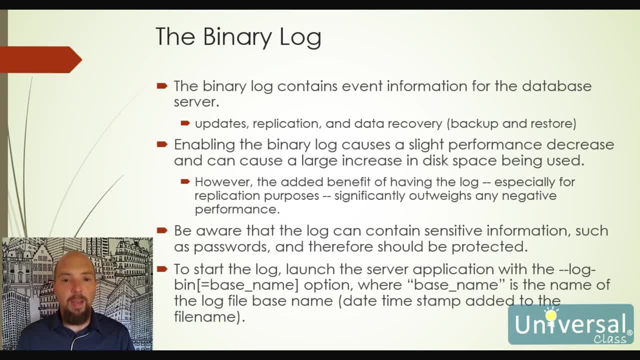 to it. So what I'm going to do with this log is that I have the ability to completely reproduce our entire database. So what I'm doing is I'm looking at the binary log and, since, whenever our last backup occurred, all the stuff that's in there is all of the statements. 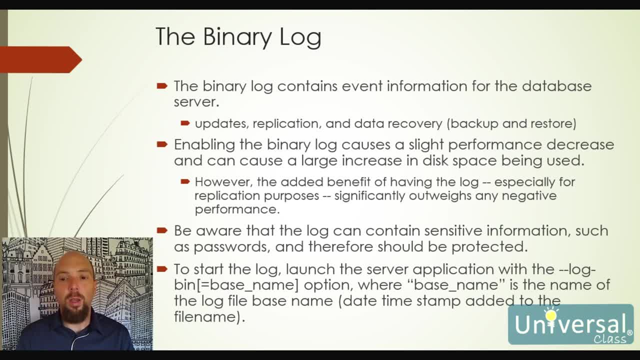 that have actually been issued. So what I can do is I can take that log, put it on another computer, and then that log would actually replicate all of the stuff that occurred on the one computer on the second one. Now, one thing you need to be aware of is that 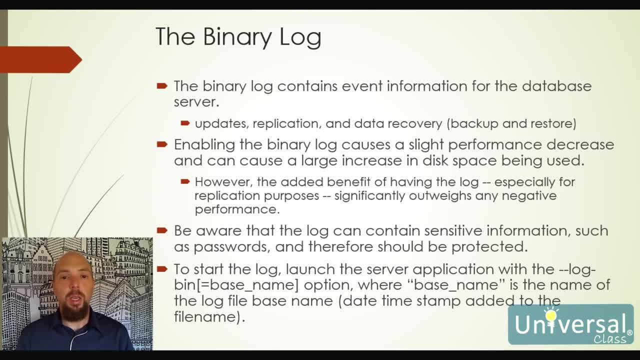 the binary log is going to contain sensitive information. It will have things like usernames and passwords in it. It'll have all that kind of information in a log that anybody can get a hold of. So you need to make sure that you protect this file. Make sure it only has. 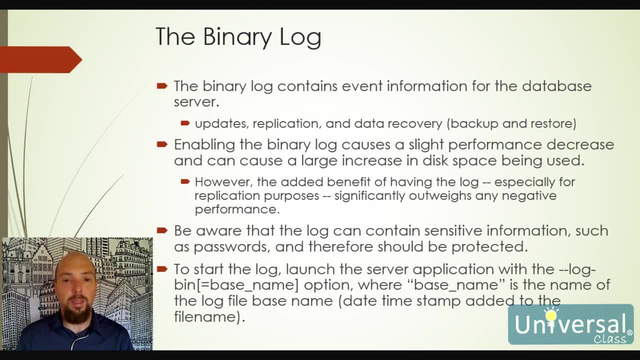 permissions for the binary log, For the people that actually need to be able to read the contents of it. you're going to set file permissions on it. So to start the log, what you're going to do on a Linux machine or a Mac is to simply start the MySQL process with the minus minus log dash bin and then 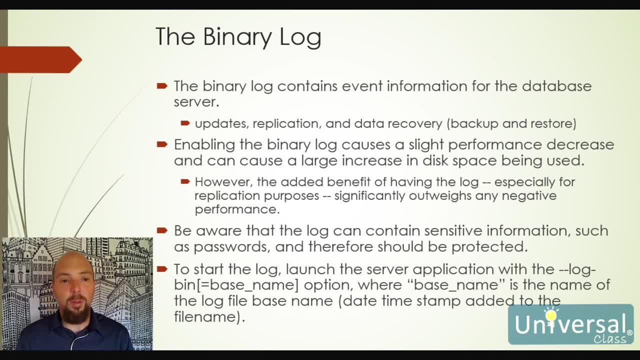 give it some sort of name. We call this name a base name. Essentially, what the base name is is going to be the name of the computer. That way, what we do is, when we replicate the data out, we know that this particular log file is going to be the name of the computer. 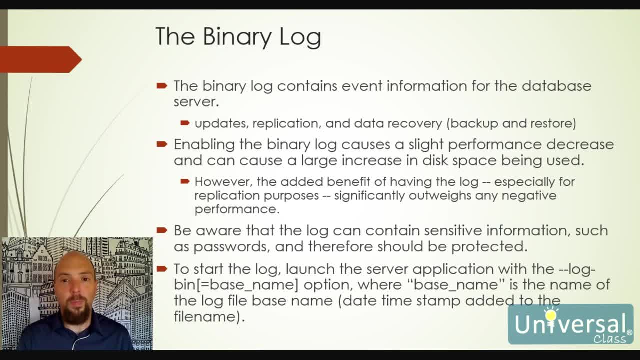 That way, what we do is, when we replicate the data out, we know that this particular log file came from this particular computer. Then what the system will do is it will add either a sequence number or a date time stamp, depending on which version you're using. 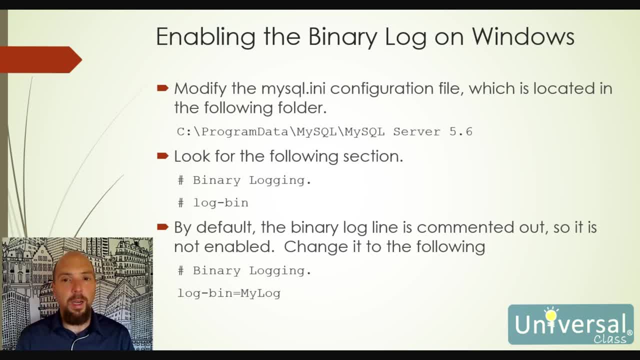 To enable the log in Windows, we actually have to modify a configuration file for MySQL. The configuration file is located under Program Data MySQL MySQL Server 5.6.. What we're looking for is in the configuration file. You need to simply enable the log. What I'm looking for is a section that looks like this: 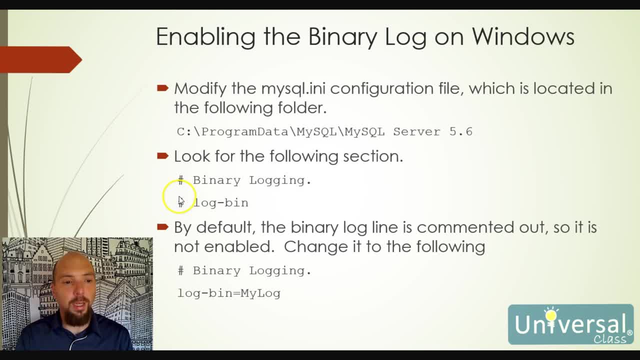 It says binary logging By default. if you notice, there's this little pound sign here. The pound sign means that this is a comment, which means it's not enabled right now. If I want to enable it, then what I have to do is to remove the pound sign and then we're. 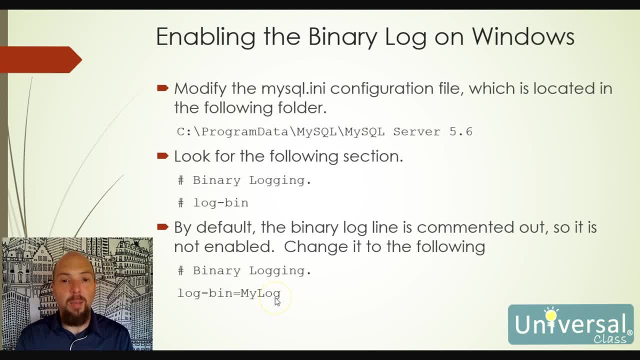 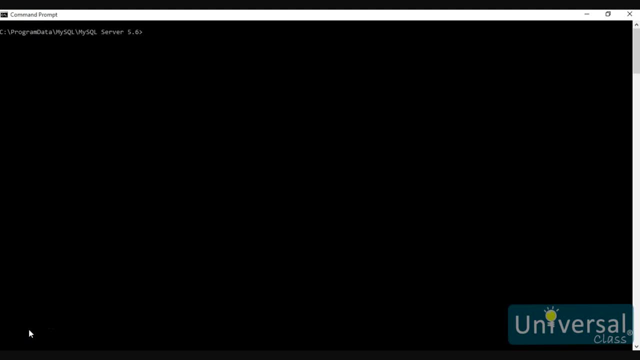 going to say equals and then whatever we want our base to be, That way we're putting the name of our computer here. All right, I'm at the command prompt, I am in the Program Data MySQL, MySQL Server 5.6 folder and if I do a directory I will. 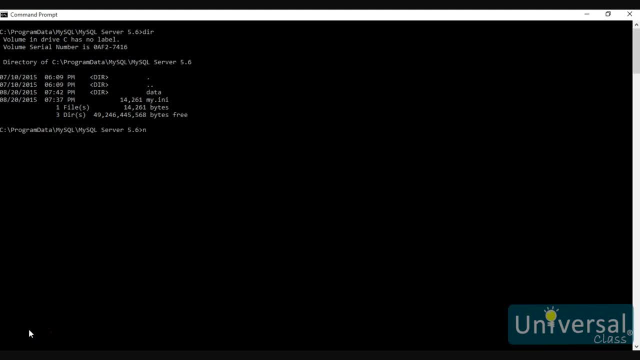 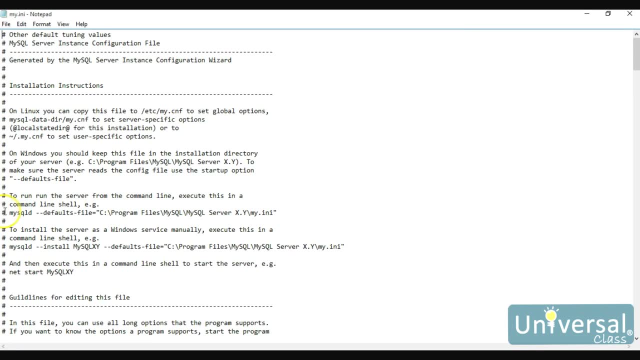 see that I have a file called myini. So what I want to do is I want to use Notepad to open myini, and this is what that file looks like Now. it is a configuration file. The pound signs over here they mean that this is a comment, which means that this actually 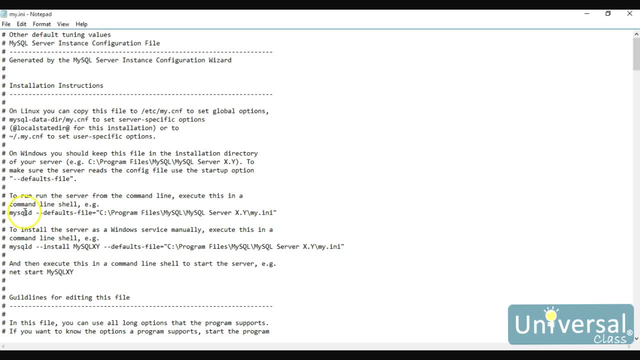 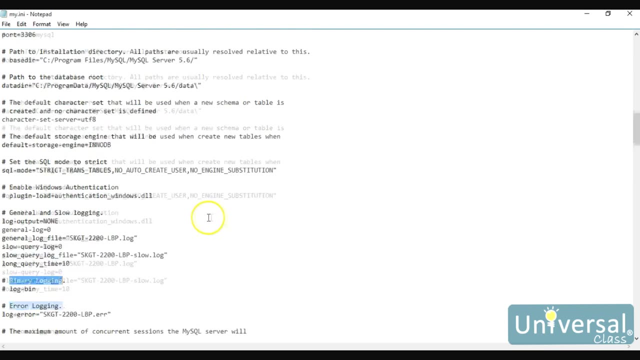 will not show. I'm sorry, will not be effective. The system will flat out ignore those. So what I'm looking for is a section that says Binary Logging. So the easiest way to do that is to find it. So I'm going to do Control F to find Binary Logging, and here's the section that I'm looking. 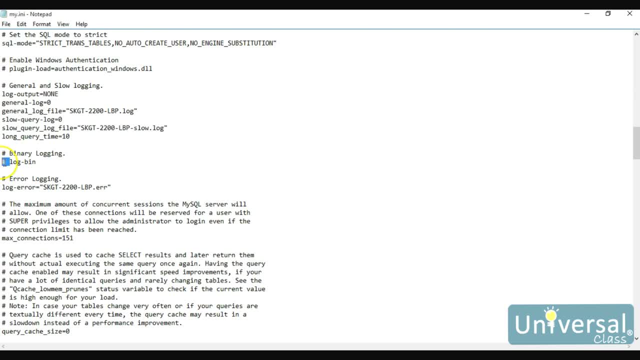 for All right. so what I'm going to do is I'm going to uncomment this by simply deleting the pound sign, and then I'm going to put an equal sign at the end. Now, if I don't put the equal sign, it will still create the log file. it just will automatically. 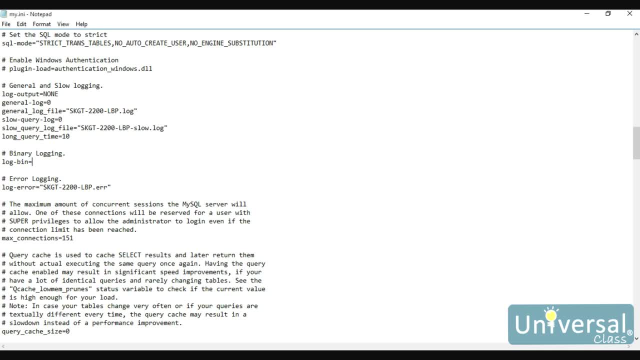 give it a name That may not necessarily make sense- That's to me. So what I need to do is I need to give it some sort of name. So I'm going to call it something like Computer Name, which in reality you would actually. 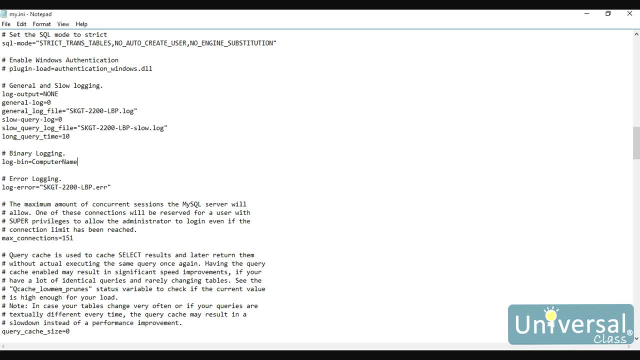 put the real computer name here. So what happens is, when I enable the logging, the files will get created and they will all start with computer name and then .0000001, and the next one will be computer name .0000002,. 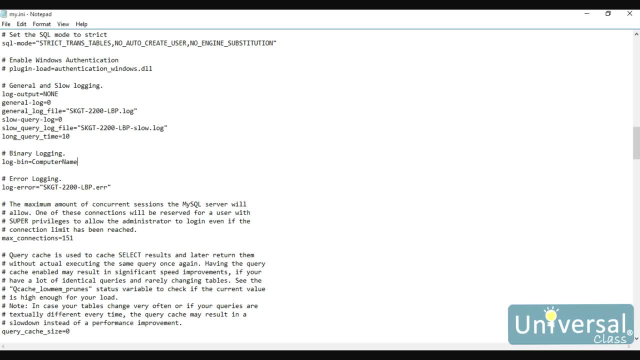 and so forth. So it makes it real easy to try to figure out which log file came from which computer. Once I have set the computer you name in here and enabled the binary log, then I want to make sure they save it, And then the next thing that I need to do is I need to stop and restart mySQL Services. 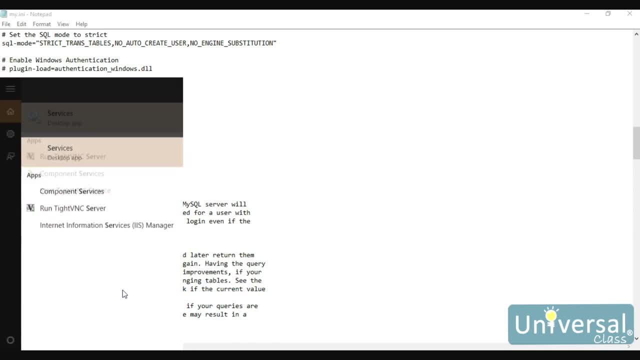 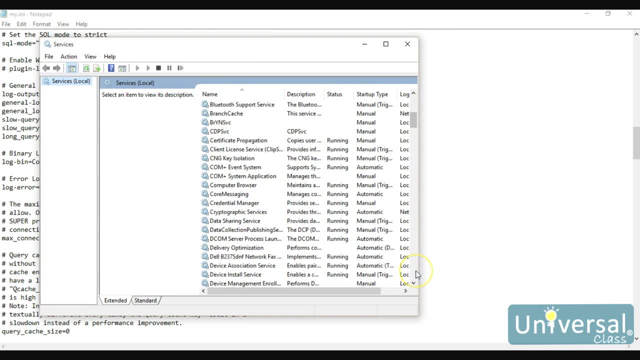 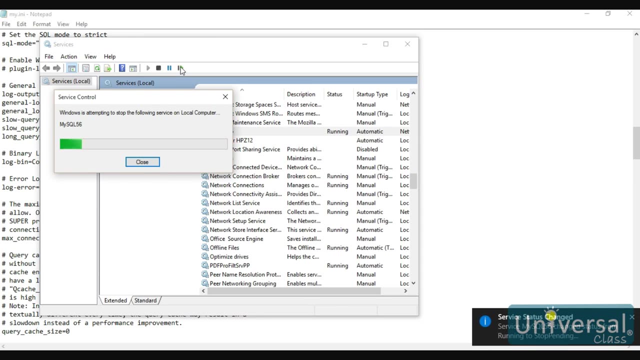 So I can do that, one of two ways. I can go to the Services Control Panel, Gentlemen For Caesar, And I can scroll down to MySQL. So here's my workbench and I can restart it. The other option is to go through the workbench itself. 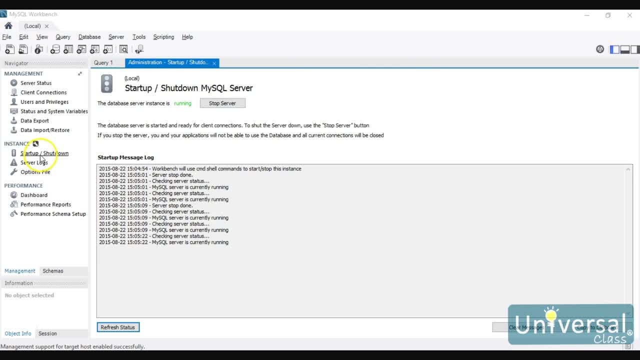 These messages and I can actually come in here to management to start up, shut down, and I can stop and restart it right here. So I don't necessarily have to have the ability to get to services as long as I can get into into the management console- I'm sorry, the workbench. 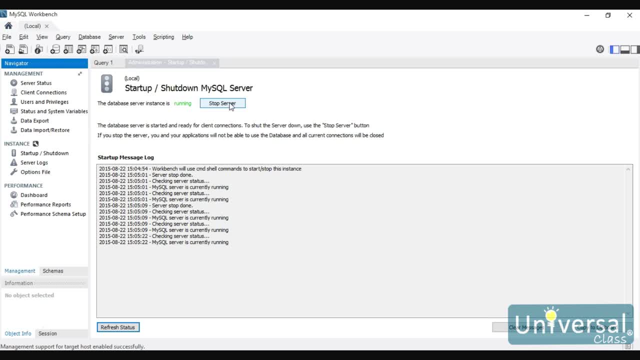 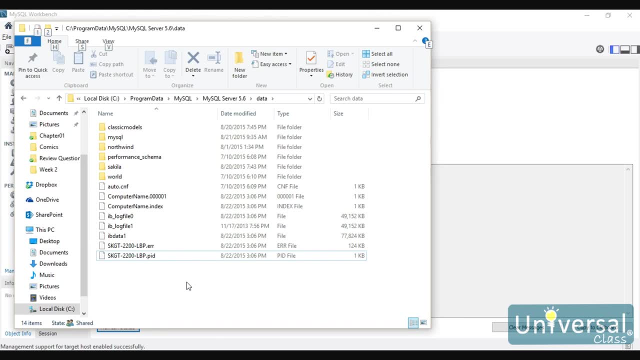 Now the problem is I have to have administrative rights of the machine. If I click it here, it will prompt me for the UAC to make sure that I have administrative rights. Once the service is restarted it will create under the program data, MySQL, MySQL server 5.6 data folder. 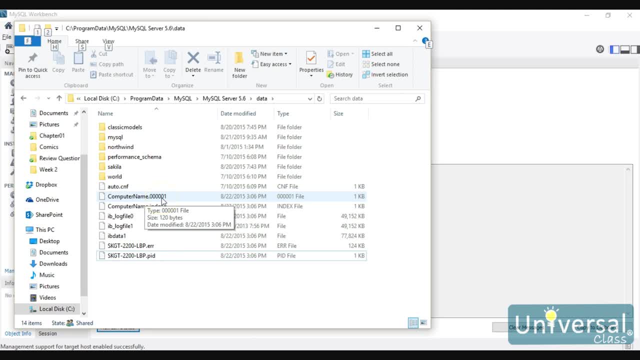 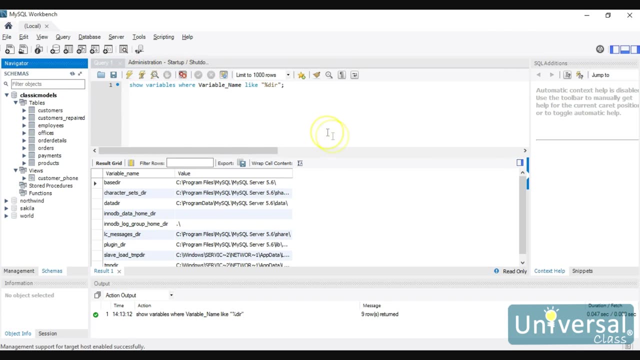 It will create our computer name, dot 00001, and what this is is the actual log, and you'll see more of these start showing up the more transactions occur in the system. So I'm going to go and go back to the database and we'll just issue some queries real quick just to get some information in the log. 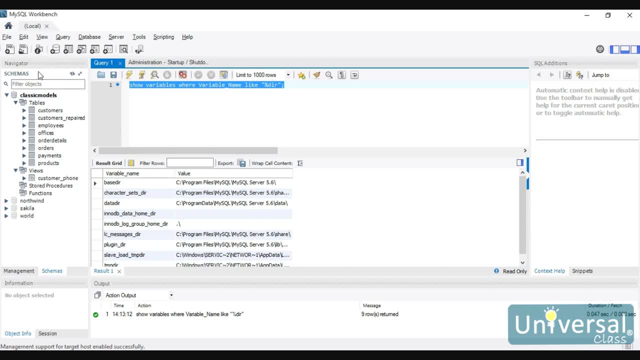 And I want to see what all stuff will actually show up in the log once I issue the commands here. Alright, so I'm just simply going to do something like select everything from- I'm sorry, classic models dot customers and we'll run this. 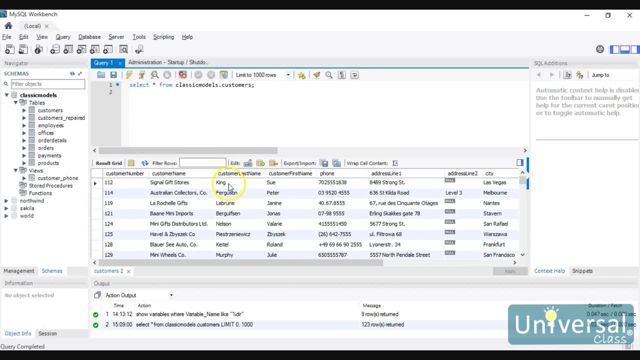 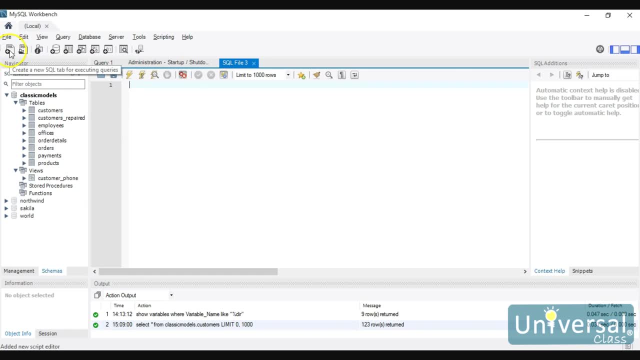 So we get everybody and I want to update the customer last name for customer number 112.. So what I'm going to do is I'm going to issue a query that will allow me to update their last name for that particular customer number. So I'm going to do an update and I'm 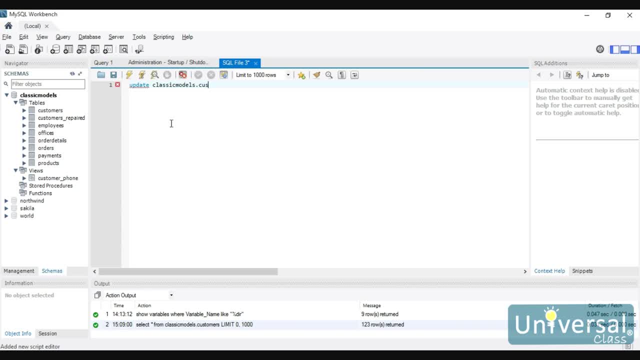 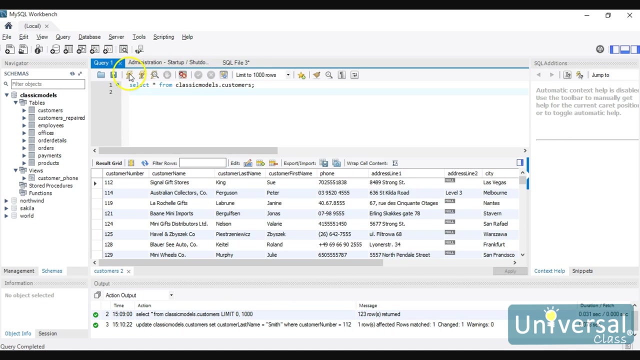 updating classic models dot customers. We are going to set the last name- see customer last name- and we'll set that equal to Smith and then where the customer ID customer number is equal to 112.. So I'm going to perform that update statement. so now, if I come over here and refresh, he's now Smith and so now the intention is to see all of these transactions in the log file itself. 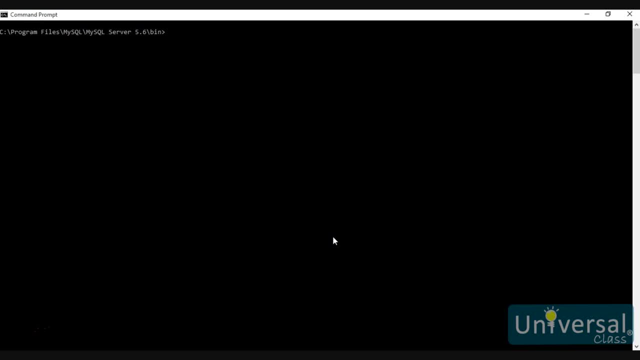 So to be able to see the contents of that log file I need to be in the binaries folder. so it's program files, mysql, mysql server 5.6, bin, and the program that I want to use is mysql bin log. And what this program will do, is it allow me to look at the contents of that log file? 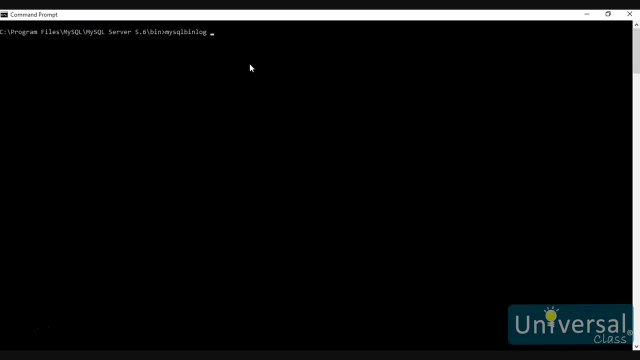 Now, by default it is stored as a binary file, which means I can't just look at it in the text editor. I have to have this program to look at. So what I have to do is tell the entire path to get to where the files located. so that file was located at program data. 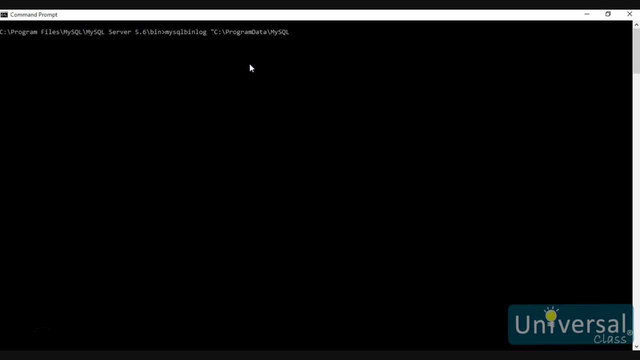 And there is a space in this, it has to be inside of quotes. so mysql, mysql server 5.6, and then it's under data and it was called computer name: dot One, two, three, four, five, zeros one. And now what this will do is it will show to me the the contents of that file. 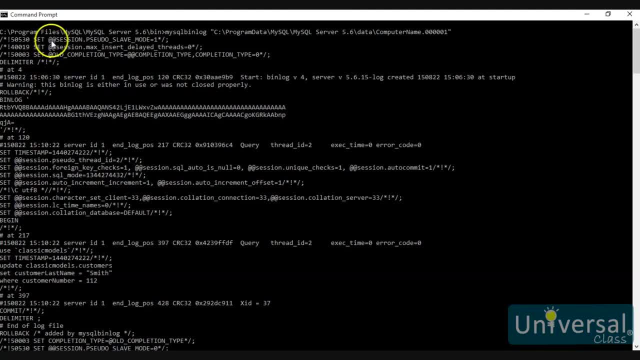 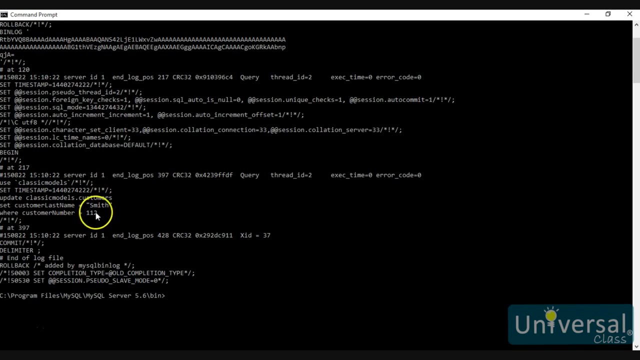 So what I can see is I can see all of the stuff that has occurred in that log file. so it's set a session number for me. It's logging other information. it actually created the log file and if I come down through the list here, I can see where I actually issued the command to update that particular customer number. 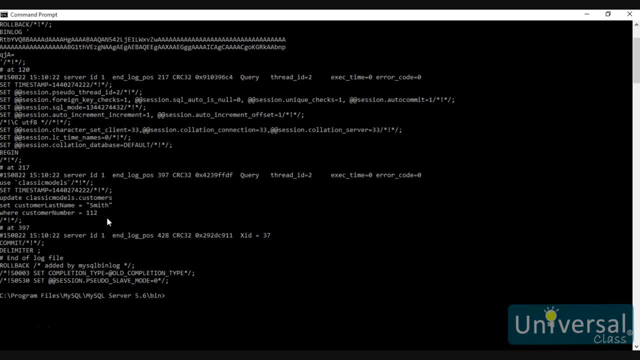 So you want to be real careful because this information is not necessarily plain text, but anybody has this program can open up this file. So now one of things: you'll notice those. there's also something here says server ID and we'll use this in a leader lesson for replication, because each server will get its own ID number. 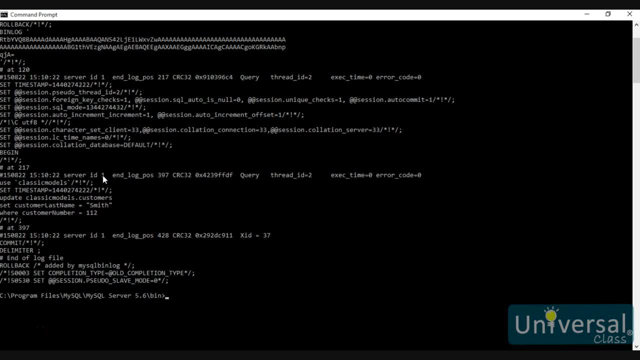 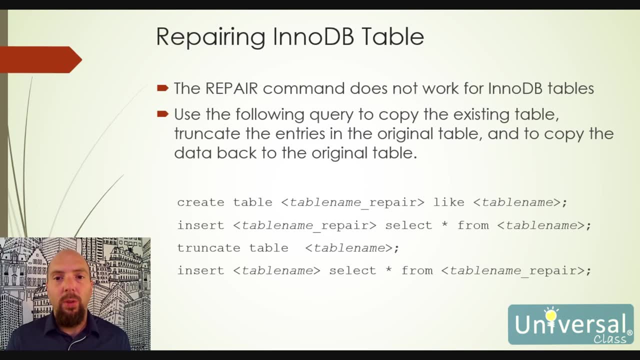 And it will allow us to be able to get information for from one server to another and be able to replicate information In A T Y W S T T S. In a prior lesson I told you that you cannot use the repair command for NODV tables. 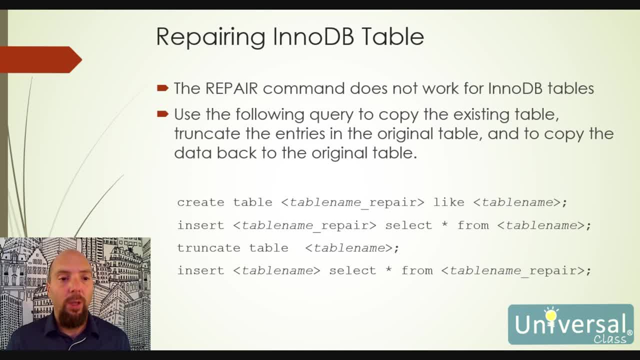 The repair command only works for MyISAM. It does not work for NODV. So what we have to do to do a repair of a table is we have to make an exact copy of the table. copy all the data from the table to the new table. delete all the contents of the original corrupted table. 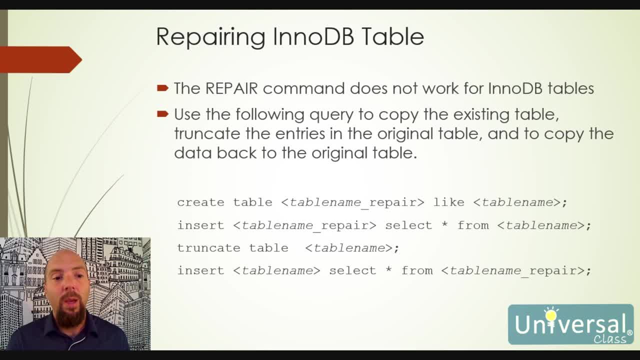 and then try to insert the information from the repair table back into the original table. It seems kind of convoluted, but it works, except for what happens is if we have a record that's actually corrupted, then we'll have to insert so many records at a time until we can find the corrupted record and just simply not insert that one. 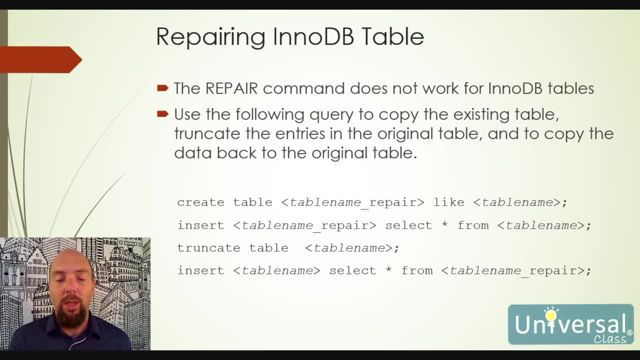 So if this works, great. If it doesn't work, you're going to have to do this, maybe 100 records at a time, 10 records at a time, 5 records at a time, and so forth, until you can narrow it down to the one that's actually corrupted. 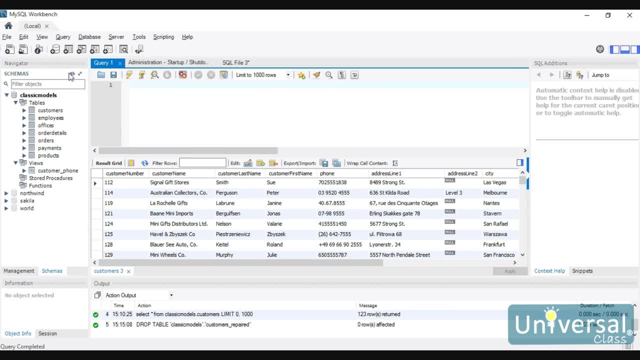 All right. so what I'm going to do is I'm going to pretend that my customer's table became corrupted and that I need to repair it. So what I'm going to do is I'm actually going to issue four commands. I could do these all at one time if I wanted to. 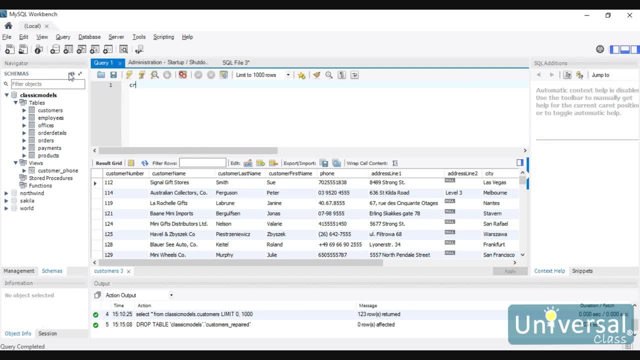 but I'm going to do them one at a time so you can see what they're like. I'm going to create table and what I'm going to do is just simply make a table where it's the name of the original one and then put an underscore- repair or something else. 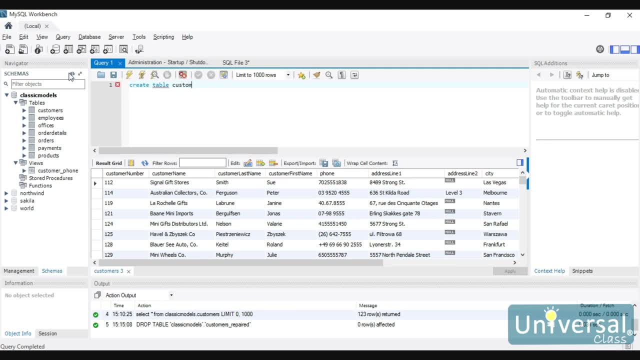 I'm going to do that afterwards so that I know it's a repair table. So I'm going to say customers underscore repair and I'm going to copy it from the customers table. So it's going to be like customers, And so what this will do is it will actually create another table over here called customers repair. 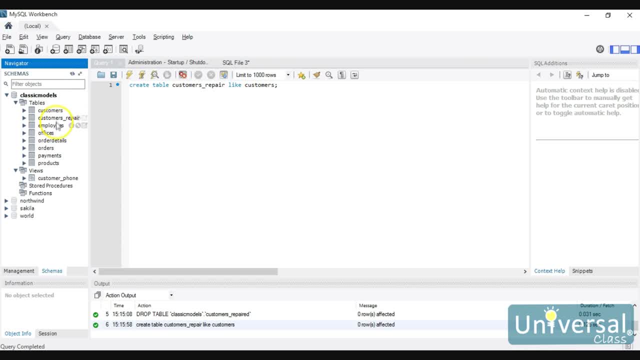 And the intention here is that I can take all the stuff that's in customers and put it into customers repair. So if I were to, if I were to look at the table for the customers repair, it's going to be the same things but the table structure. 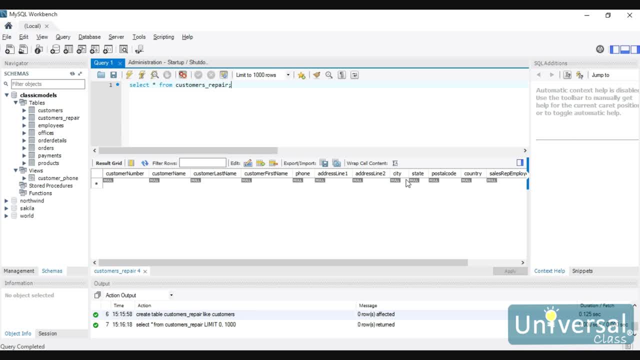 The table structure is there, but there's no data in it, Because all I did was by using the light command. I just simply took the structure of the table and constructed another table with that same structure. All right, So the next thing that I want to do, I've already created it. 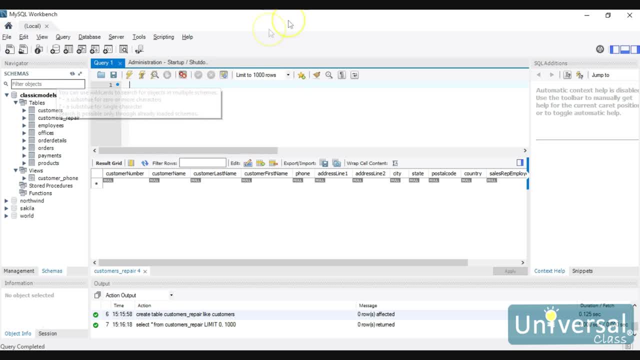 I modeled it after the original one. Now I want to take all the information that's currently in the customers table and stick it into this repair table. So I'm going to insert things into customers, underscore repair from a select statement. so I'm going to select everything from customers. and so now what this is going. 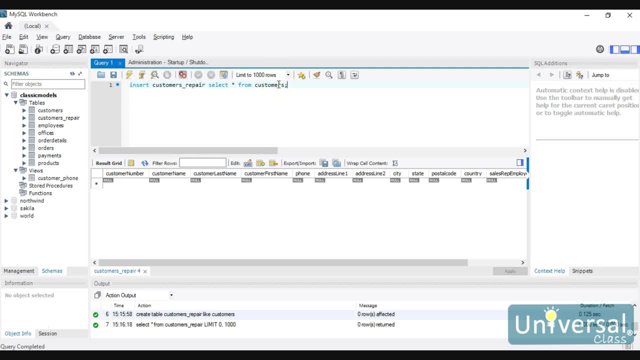 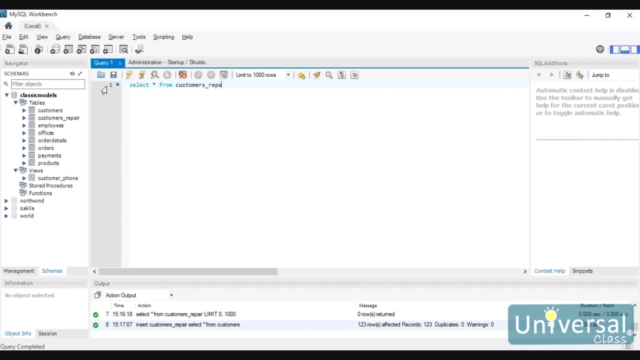 to do is it can take the select statement, select everything from customers. it'll load it in a table in memory and then it will insert all of that stuff into the customers repair table. so run that now. if I select everything from customers underscore repair. now we have data in here and the 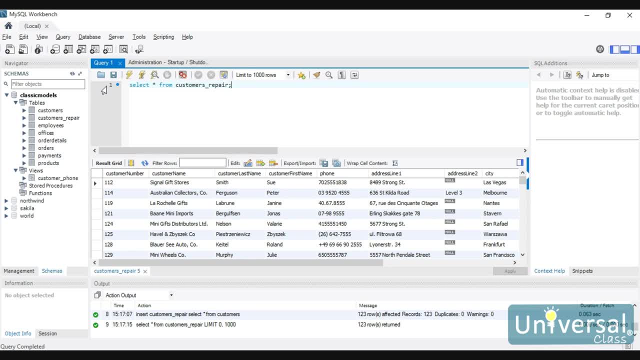 data here should match the data that's in the other table. now what you may encounter is that you got errors, and if you get an error and it says that there was an error at record such-and-such, then what you would have to do is limit. 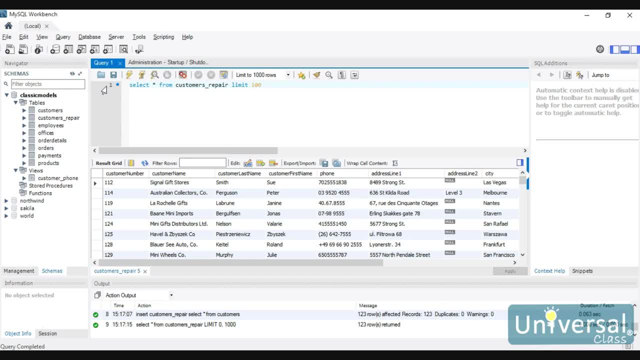 the number of records, so maybe you only do a hundred at a time, and so what this is going to do is it will copy the top 100. you're going to do is it will copy the top 100. now what would happen is, if this is successful, then you copy the top 100. 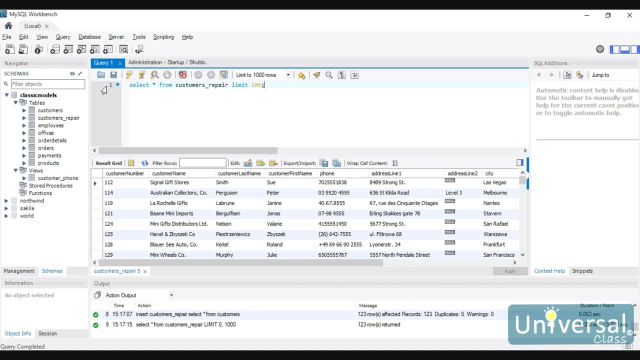 then you delete the top 100, then you copy the news, the new top 100 and delete the top 100. you have to keep doing this, so it may take a little while. if one of the records is corrupted, you would have to actually limit it to this amount of. 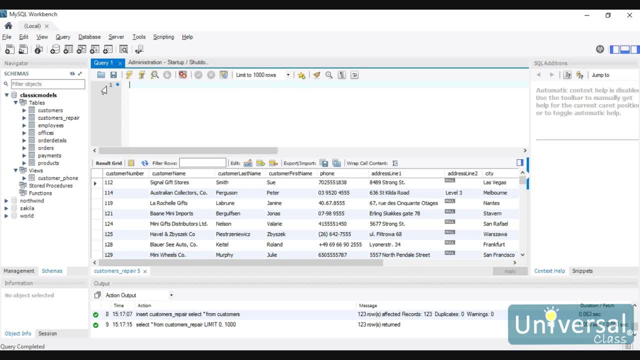 tape of information. okay, so I want to get rid of the data that's in the customers table. right now, we have all the data still in the customers table, so what I want to do is I want to get rid of the data that's in the customers table.